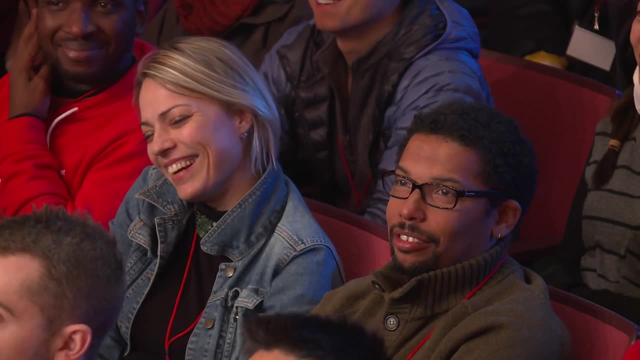 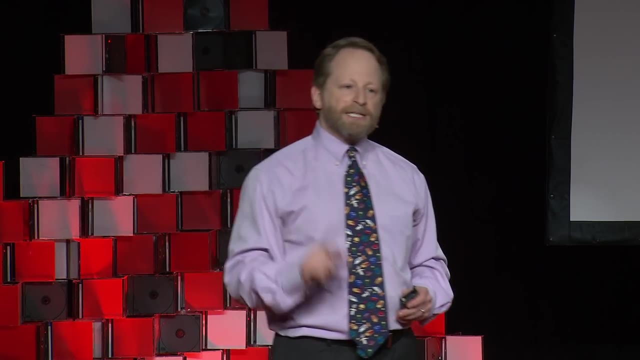 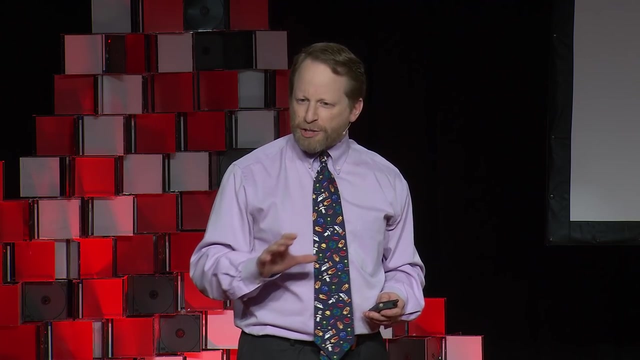 Hello Grandpa. So it's kind of interesting. If you visit any kindergarten anywhere in the world, anywhere, you'll see the same thing. You'll see children using all of their senses to learn about the world around them. Small children are great learners. They look at everything, they listen, they touch things, they smell things. 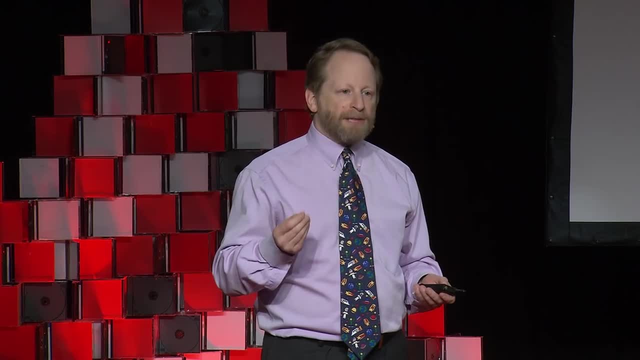 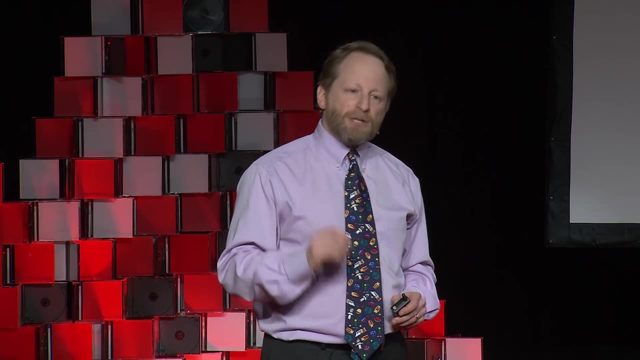 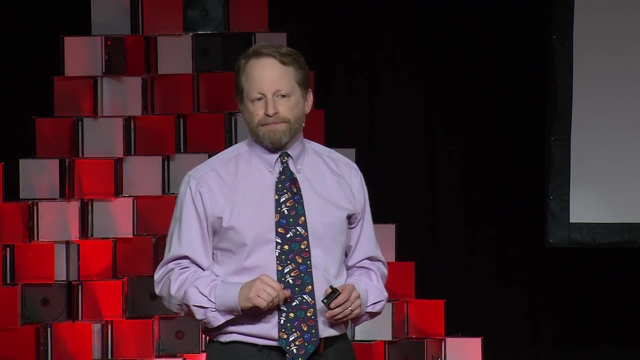 Small children even put things in their mouths to learn about things. Small kids lick stuff. It's disgusting actually, But if a child doesn't know what something is, he or she will do anything to figure it out. It's just the way we're wired. 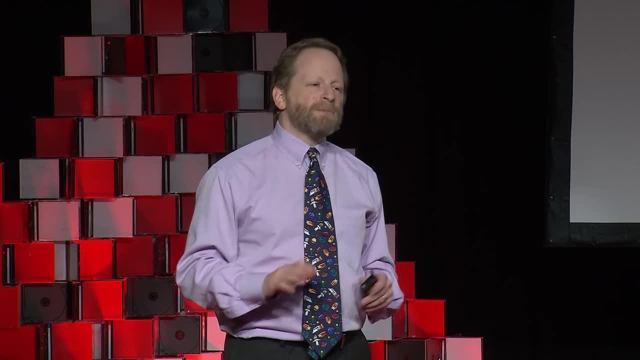 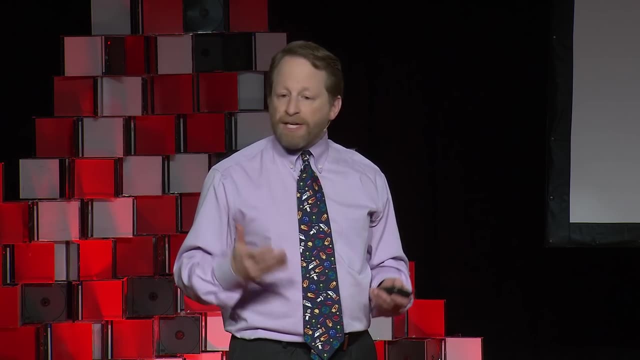 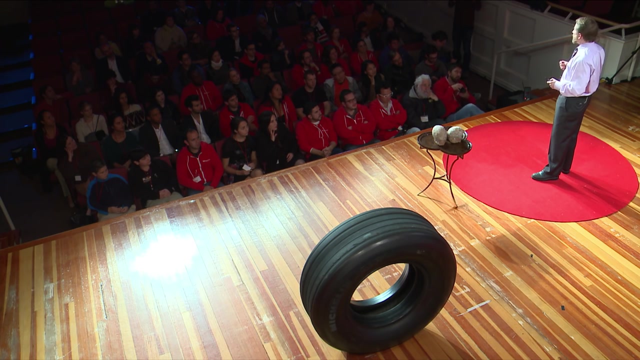 Fast forward to adulthood and you see something completely different. You see, these same formerly curious children are now adults living in a society where the average adult is less scientifically inquisitive and a little less curious than your average five-year-old child. 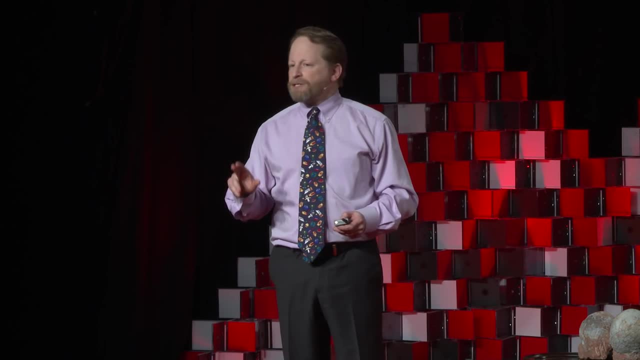 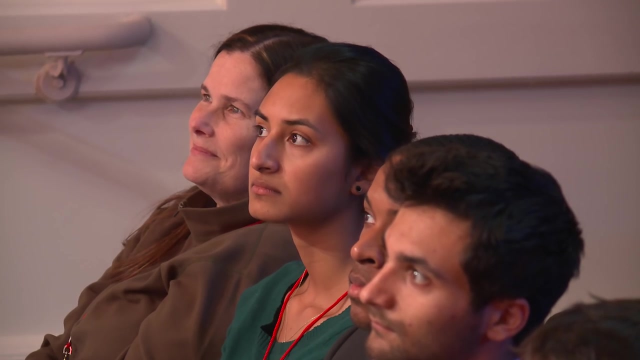 How can this be? I'm not saying adults aren't curious, because they are. What I'm saying is, at this time, at some point, we stop thinking about ourselves as scientists. I believe that if we can teach our children to keep that scientific curiosity and wonder with them as they grow up, 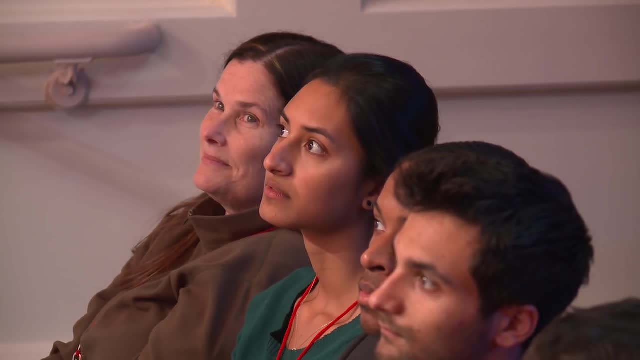 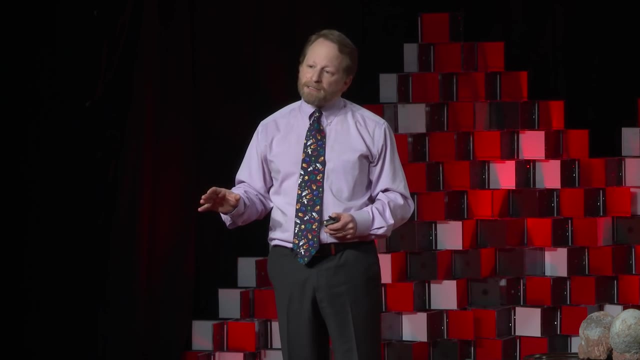 our world would be a very different place, And I think we can do it. I would like to live in that world, So today I want to talk to you a little bit about science and scientists and how we teach these things to our children. 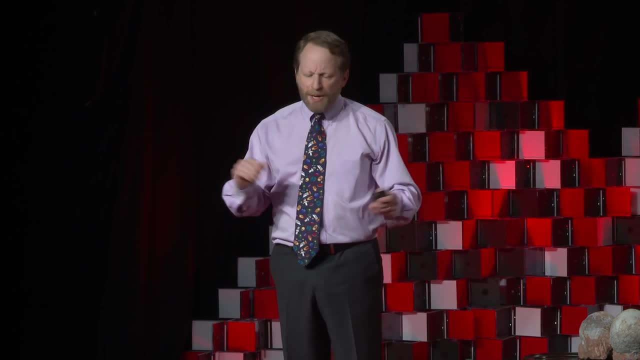 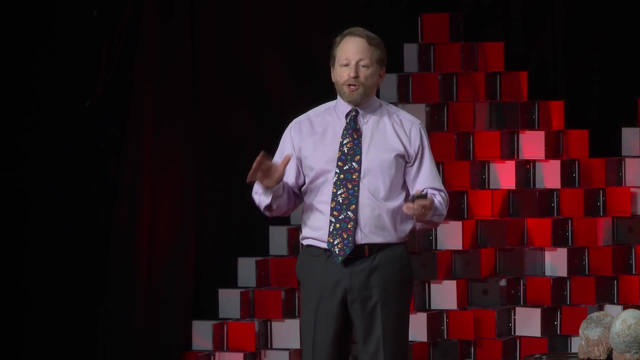 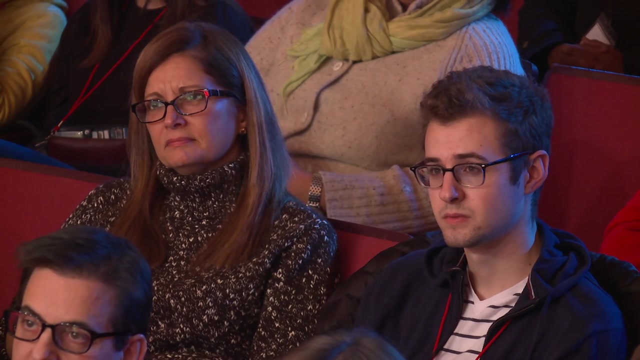 Sometimes well, sometimes maybe not so well. So let's start out talking about scientists. If you went out on the street and asked an average, normal, well-adjusted person to give you one word that describes a scientist, do you know what most people say? 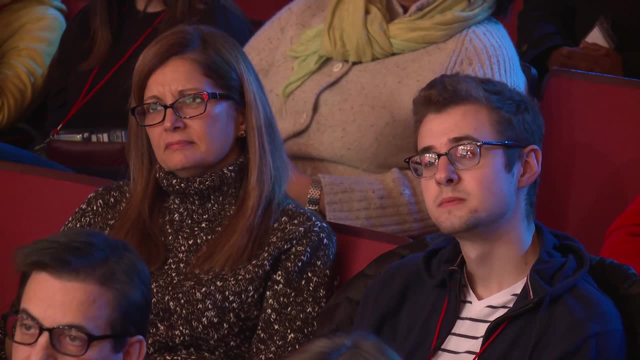 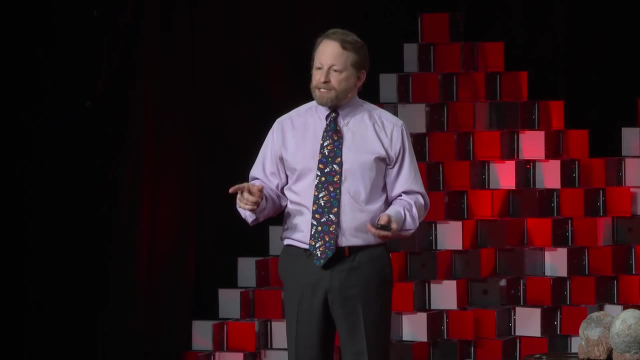 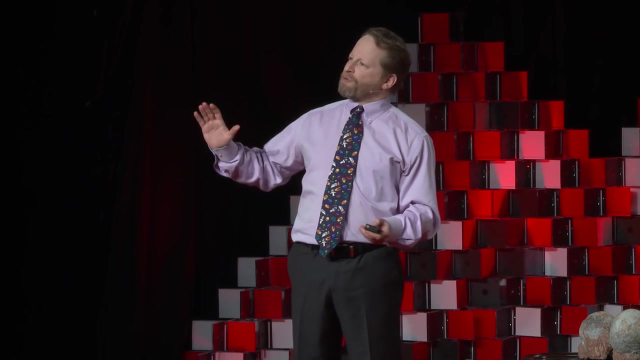 Smart. They say scientists are smart. Would you agree with that? It's not necessarily true. If you ask the same question to a normal, well-adjusted scientist, if such a thing existed, he or she would say something like: science is the pursuit of truth through experimentation. 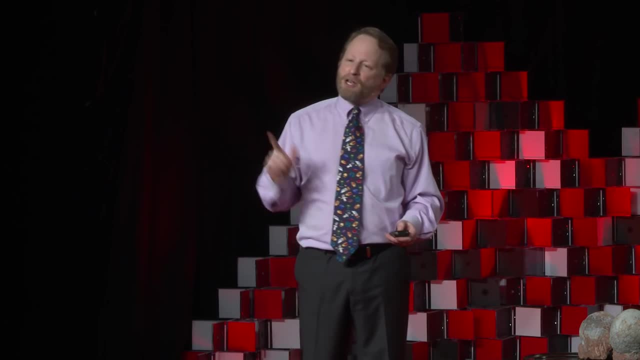 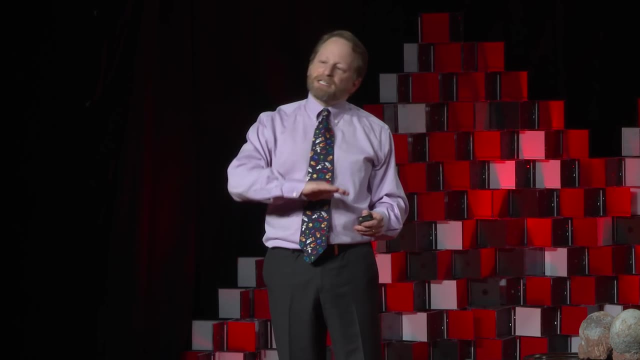 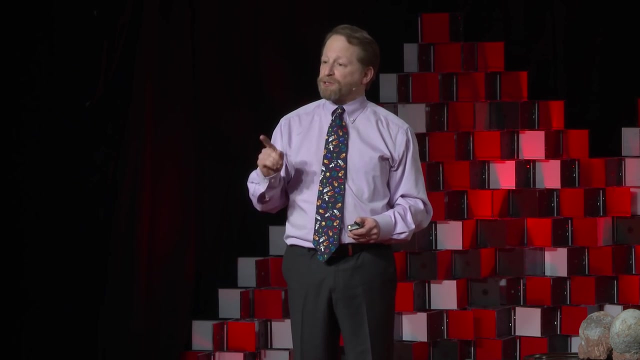 How about smart? Are you kidding me? That's not even one word. See, not all scientists are smart. It's like you know. some are some. eh, It's a distribution like anything else in the whole world. You can't tell me there aren't dumb scientists, because there are. 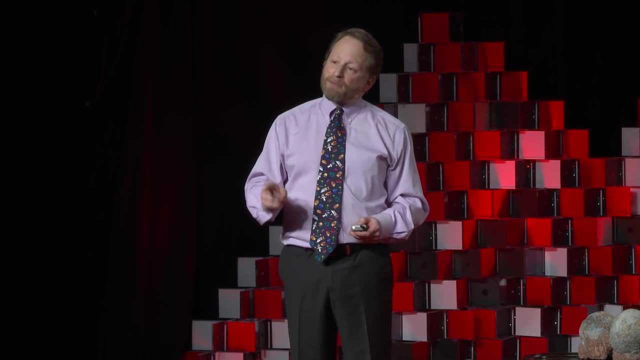 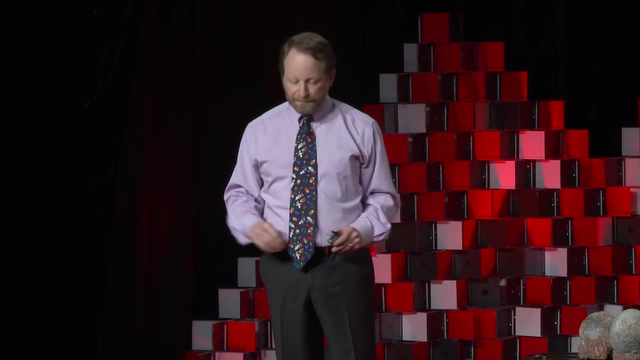 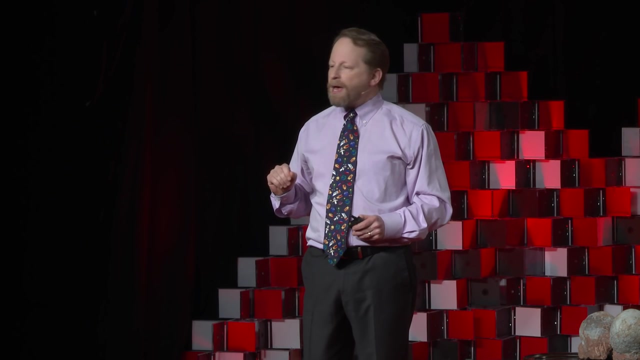 My theory is: the average person is probably smarter than the dumbest scientist. You know what that means. That means anybody can do science. so there, The secret of science is this: Scientists are very well educated, highly educated, But highly educated doesn't mean smart. 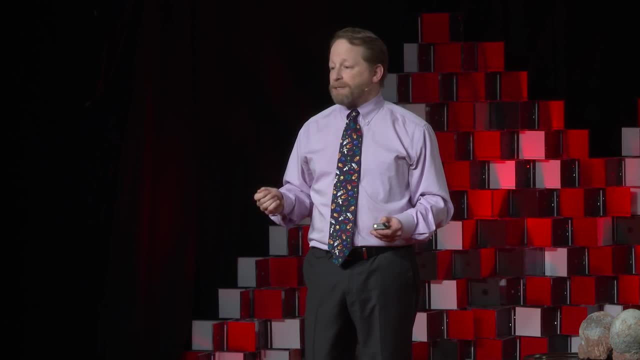 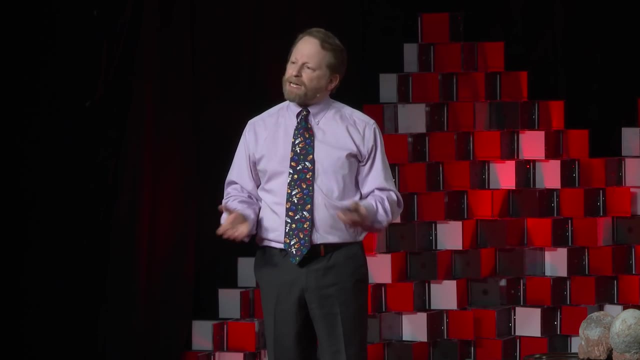 in the same way that uneducated doesn't mean dumb, Our children, when they're young, are not educated and they're not dumb. So as we talk about science and teaching, keep this in mind: Just because someone is educated doesn't mean they're intelligent. 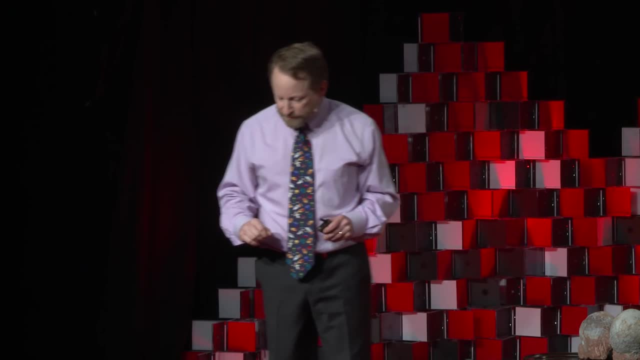 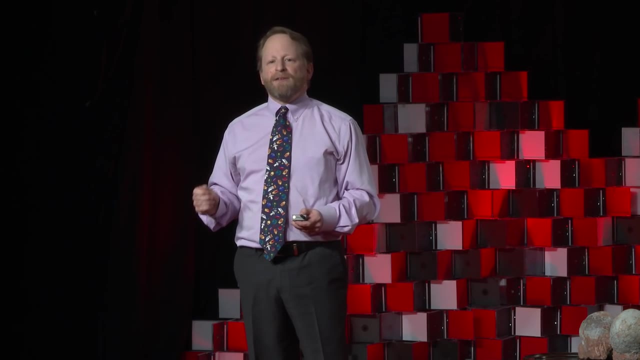 Look at all the politicians. So this sorry politicians if you're here, Here's the way it works. Science is interesting to me for several different reasons. There's a lot we can learn about in school. We can learn science at home as well. 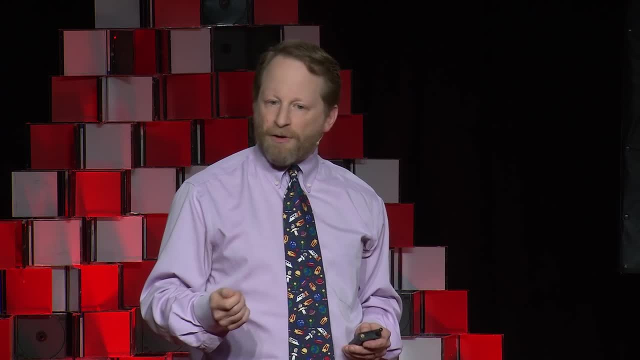 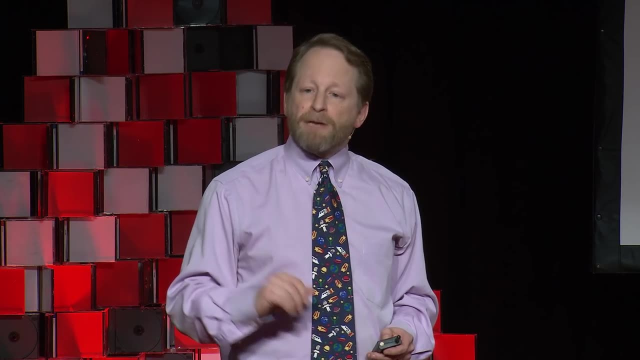 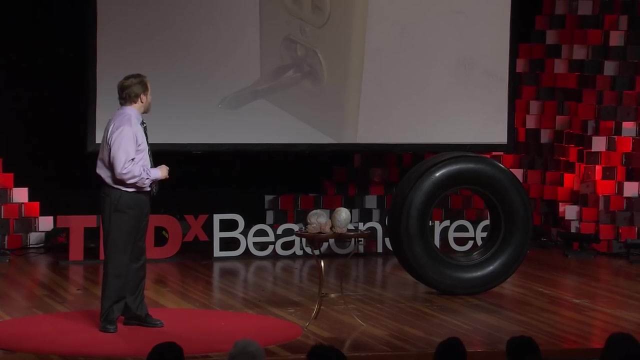 In fact, a lot of science begins when you're very young. Remember how I said, children are natural born scientists. My son, Milo, when he was five, did this fancy bit of science right here Apparently. it's a thing. Some kids do it, I never did. 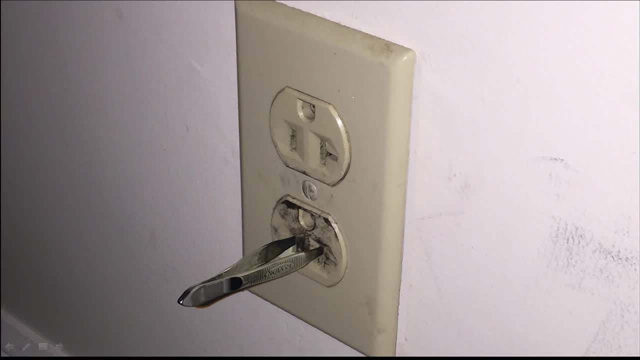 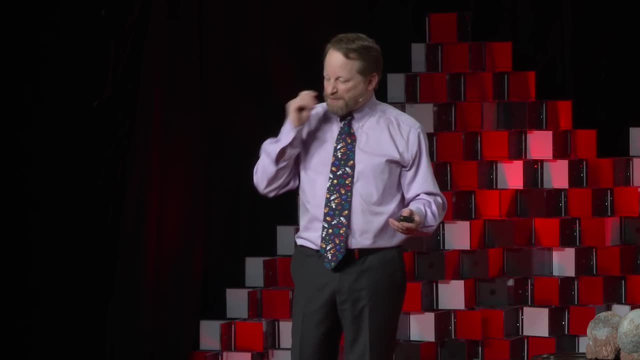 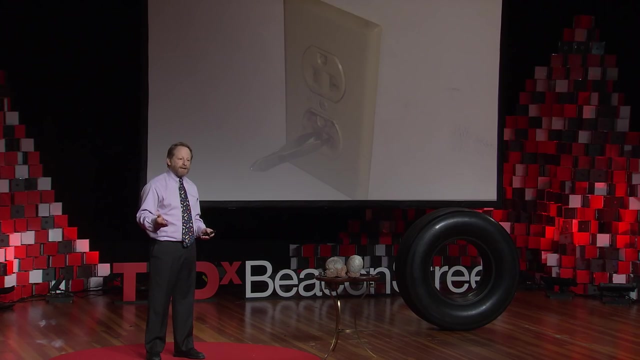 But this is real. So here's what happened: The lights went out and there was a smell. It was like a burning smell, It's true. It came downstairs and that my five-year-old son standing there didn't stop for a moment. 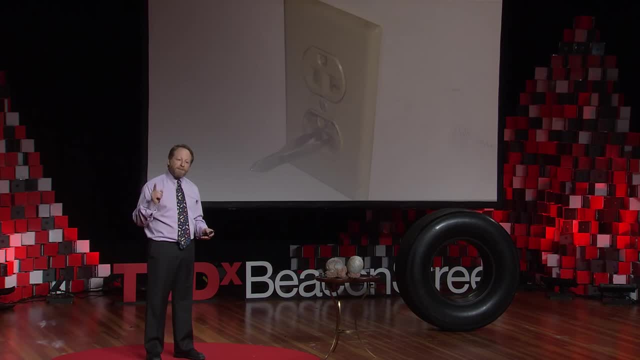 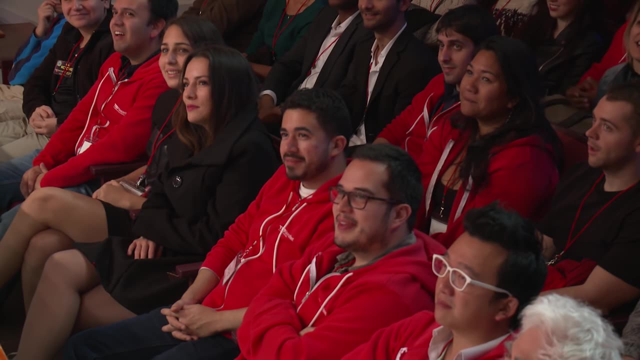 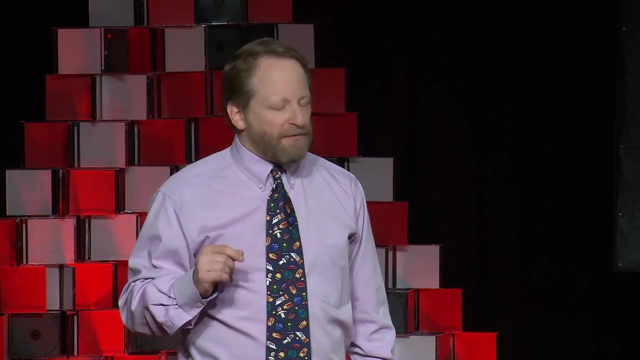 He looked up at me and he said, Dad, it wasn't my fault, I just wanted to see what would happen, And so I didn't know what to do. This is true, So I sat for a second and I'm thinking to myself. 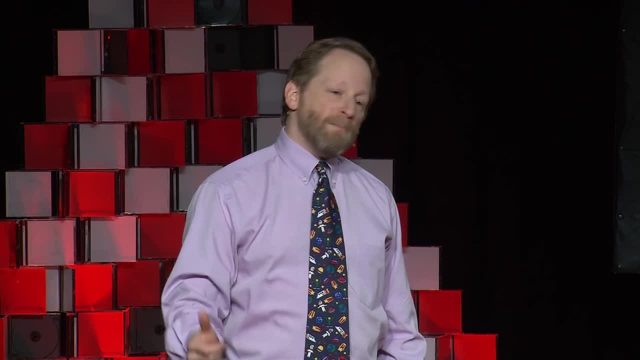 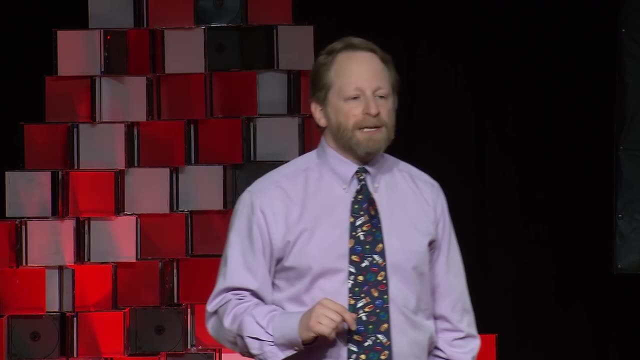 he's standing there next to a smoking hole in my wall, holding an oven mitt on the other hand, and he's telling me: it's not his fault, But you know what He was telling me? the truth He really was. It took me a second to realize it. 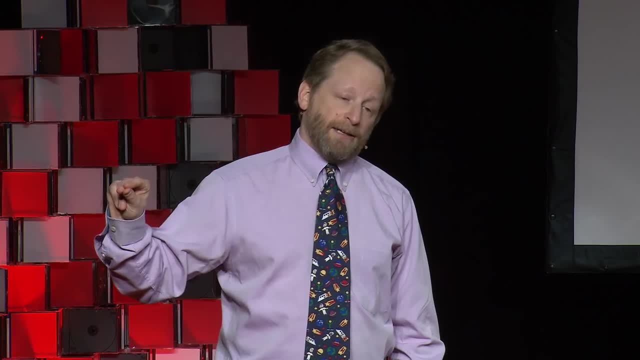 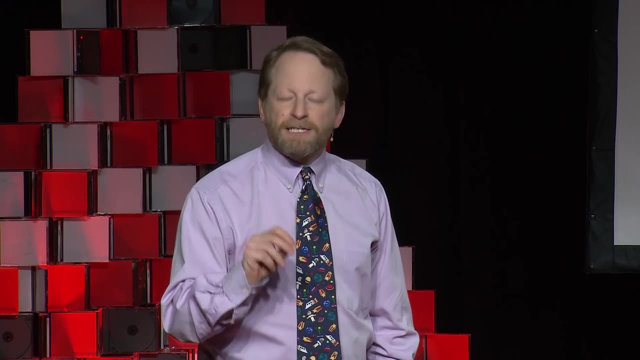 He wasn't saying he didn't do it because he did. What he was saying was: it wasn't his fault. He was curious. Let me tell you again, a little bit more slowly, his exact words. He said: it wasn't my fault. 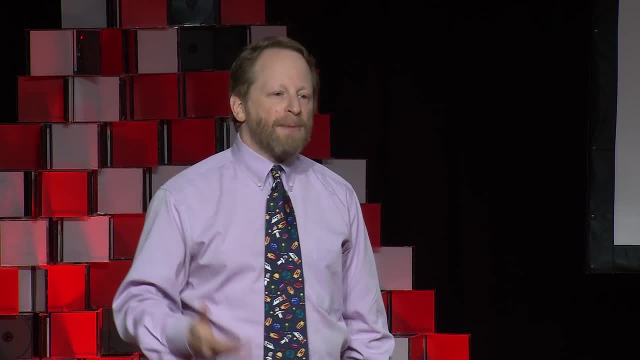 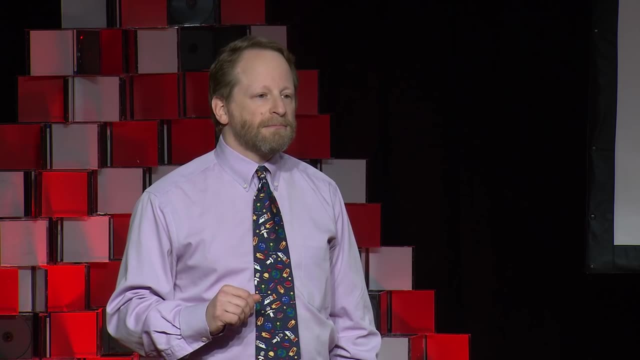 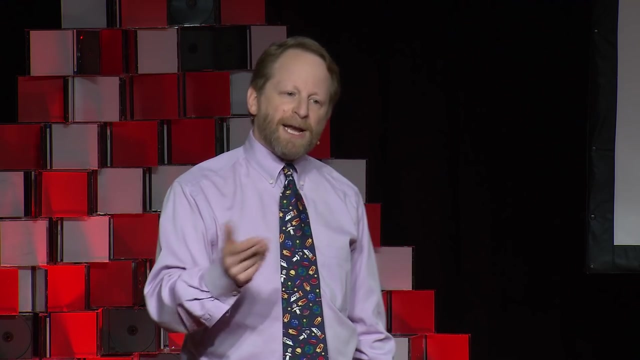 I wanted to see what happened. He was describing simple, irresistible human curiosity. It really wasn't his fault. So what am I supposed to do now? So I had two choices. I won't tell you what I did, but I'll tell you what the two choices you might have. 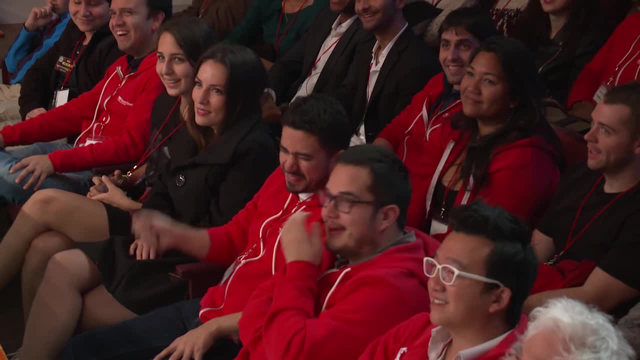 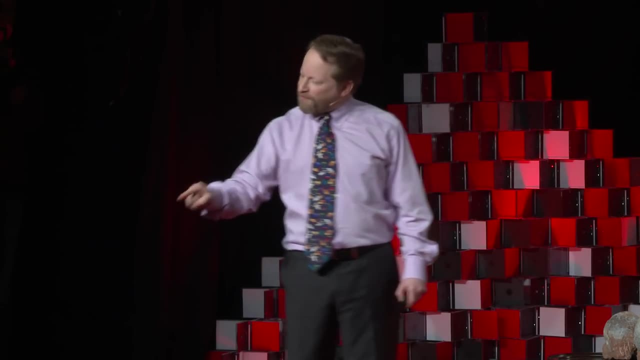 All right, all right, All right. I'll tell you what I did. But first, what do you do? You say that was the stupidest thing you ever did. I'm pointing at you: Don't you ever do that again? 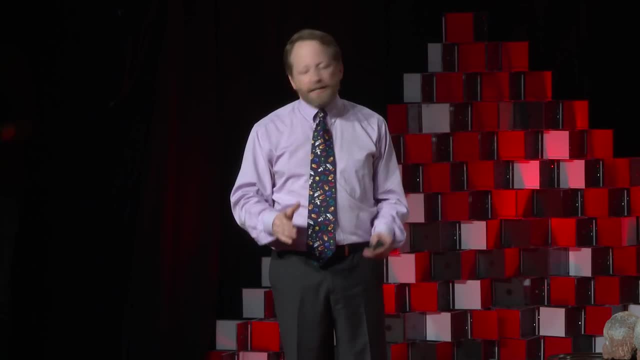 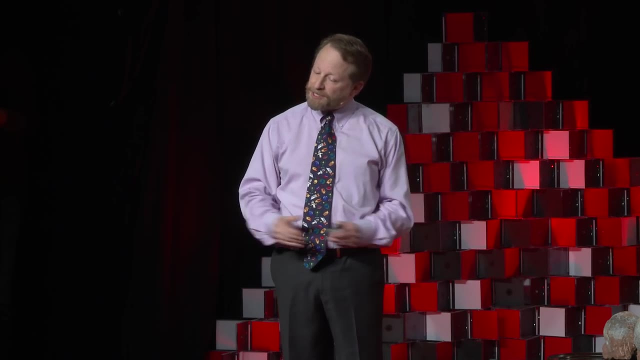 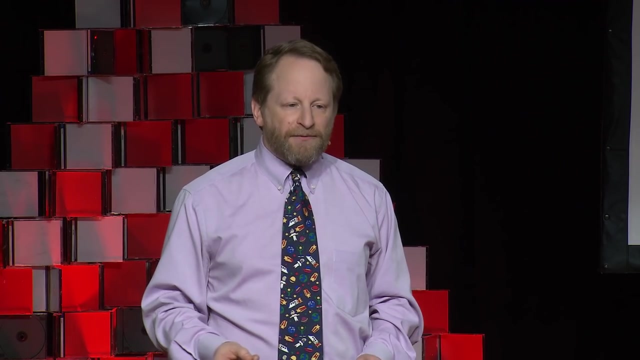 Or do you say: okay, what did you learn? What would you have said? It's a tough question. You see, we don't really have to control their curiosity to keep them safe. We have to protect their curiosity to keep them fulfilled. 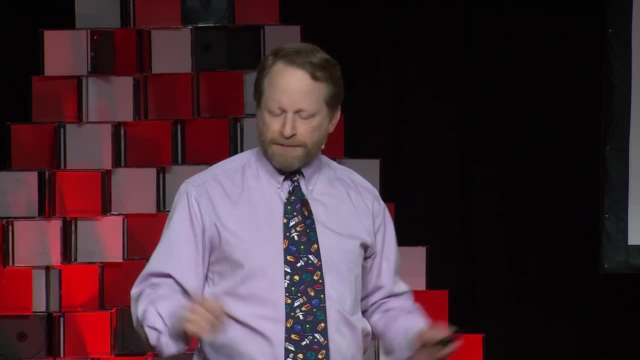 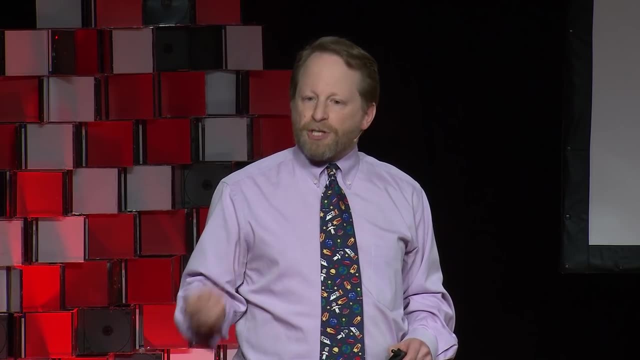 Our kids. So all I can say about that is: I did do the latter and we talked about it. The idea is, kids are curious And we learn a lot about science at home. These are moments. they're like turning moments. 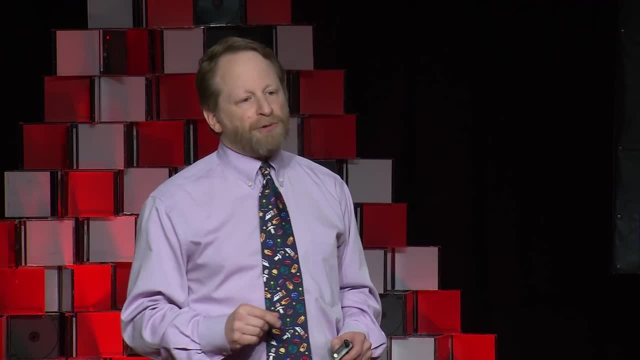 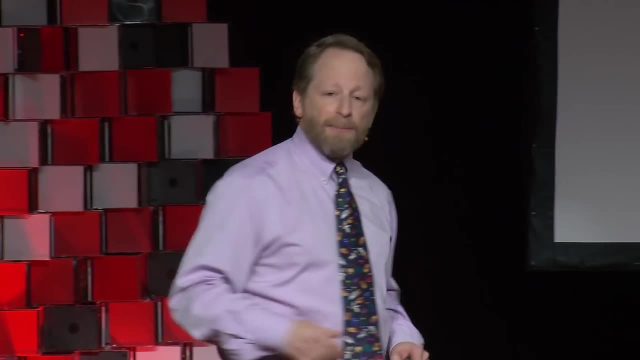 They're like turning moments. If we punish curiosity, that child will never do it again, And that would be a shame. So some of this learning happens at home. We learn about science, of course, at school as well, And schools are excellent at teaching science. 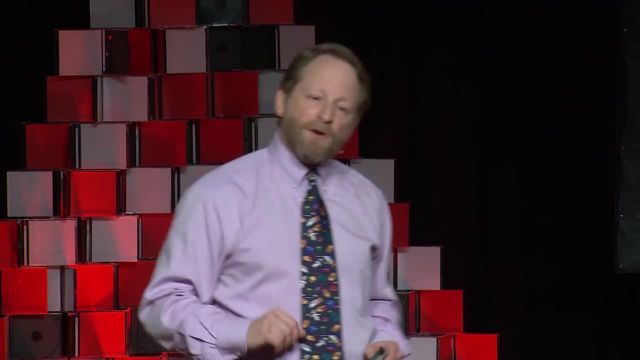 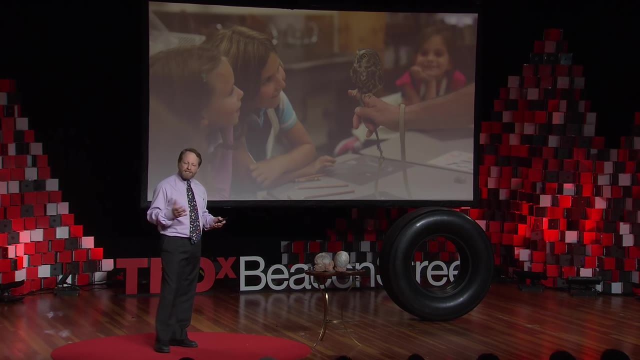 especially, especially at a very young age, when everything is hands-on, For example. who doesn't remember going and learning about science for the first time and being involved in real stuff? Students love science. Students love learning when it's hands-on. 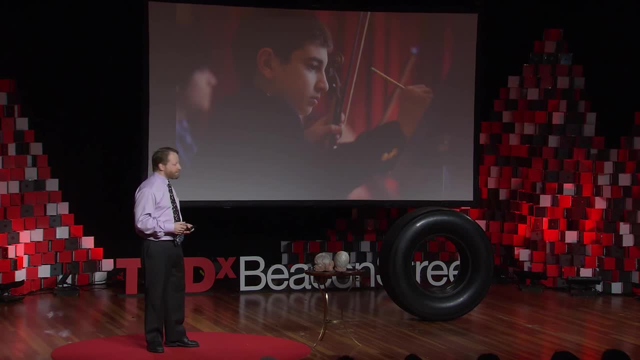 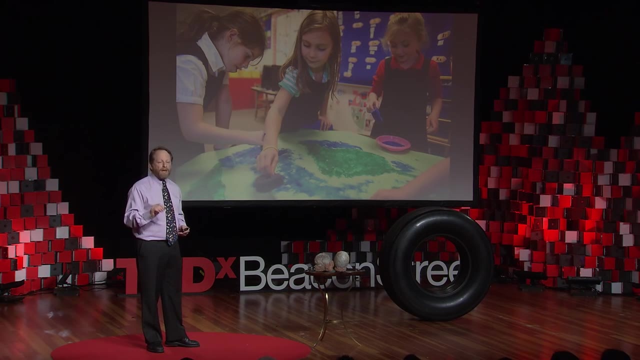 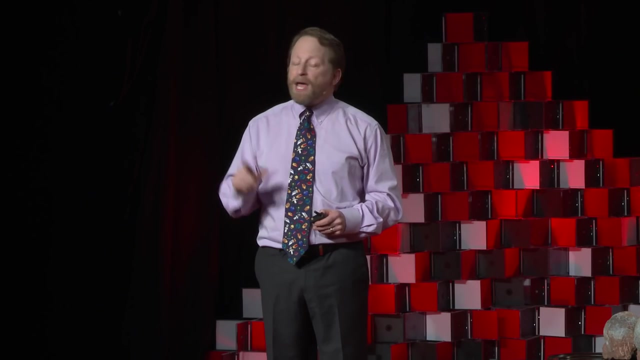 when it's real. Whether it's science, music or art, Students do best when they connect with something. So in school we learn that at a very young age students need to connect with something real. That helps in a great way. 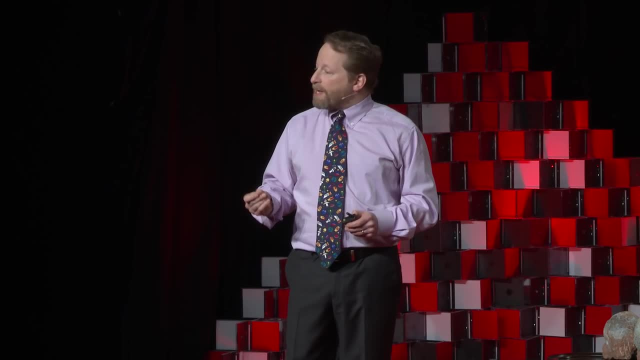 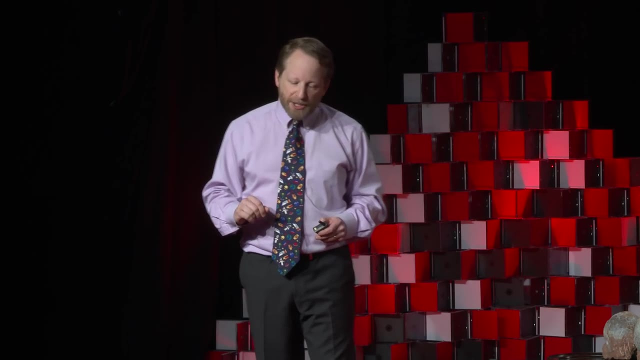 And I learned this as a teacher by going on a field trip, And that field trip was to a museum where they had a special exhibit on dinosaurs. We saw a 20-minute demonstration that was designed for five-year-old kids. I loved it. 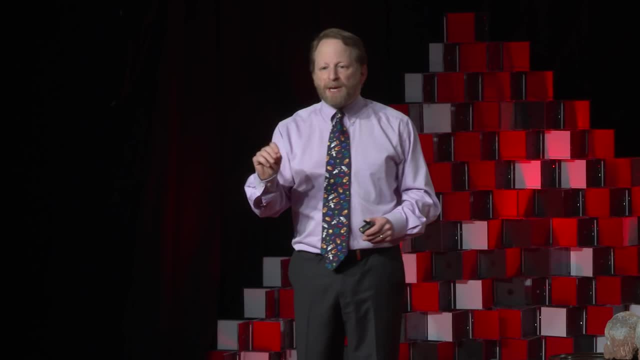 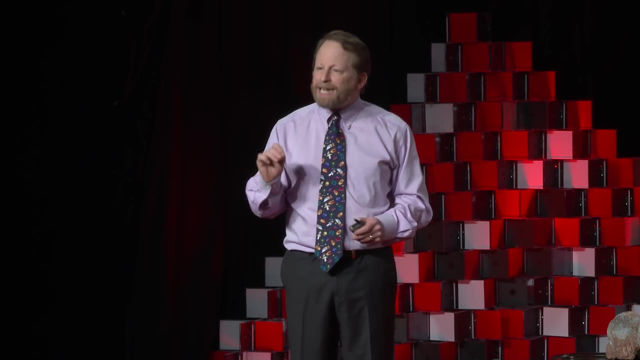 It was great. It tells you a little bit about me. The best part about it: these kids were excited because they got to touch a real dinosaur bone, A real dinosaur, 100 million years old. I thought that was exciting too. 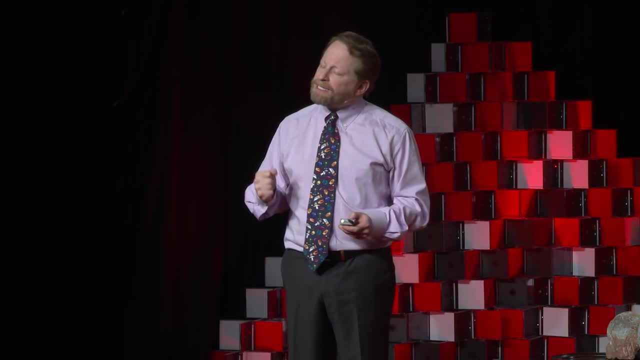 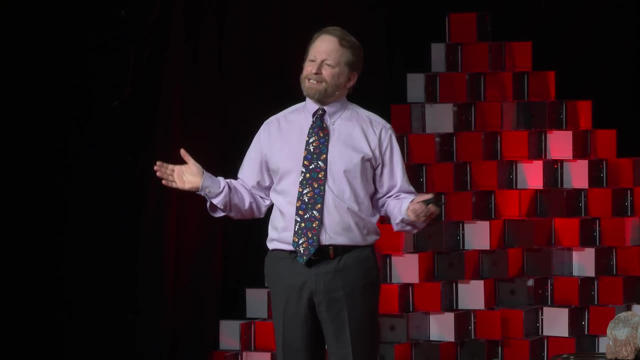 So students were learning, they were excited about dinosaurs and they got to be involved. Until at the end of the program when the woman said, oh, that's not a dinosaur bone, It's a plaster cast, And all the kids just sort of deflated. 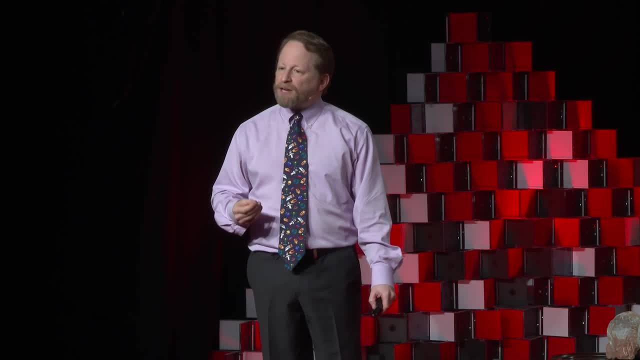 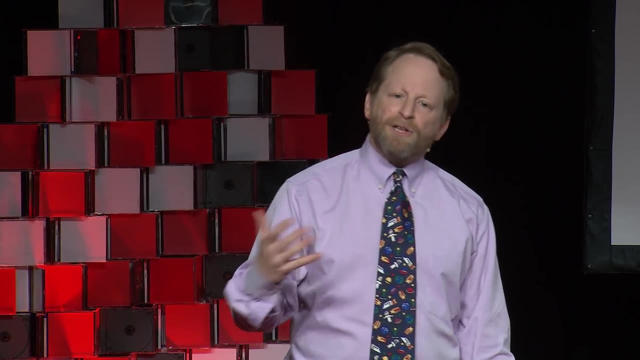 Because for them at that young age, a lot of it has to do with connecting in some way to the event. And we're no different as adults. You know, when you go to a museum, do you want to see the real Mona Lisa? 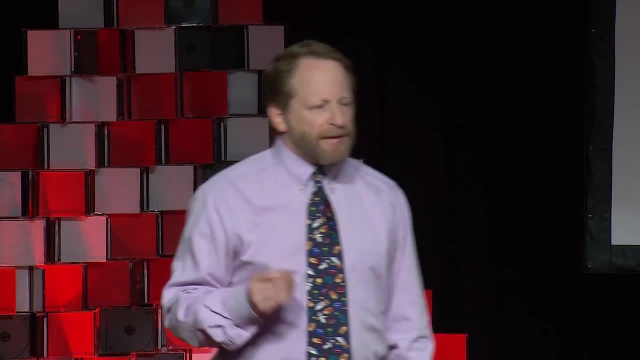 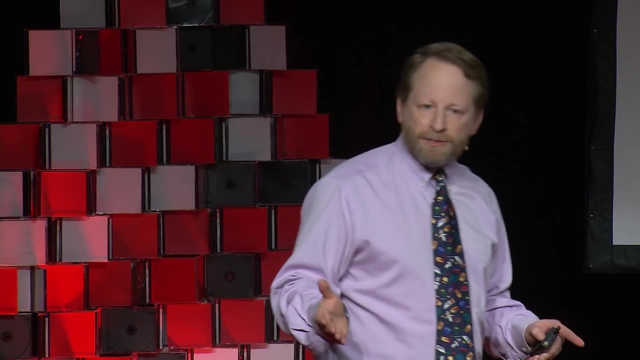 or the poster in the gift shop. You want to see the real thing. So that's when I learned that students like to learn things by attaching to an object or finding some relevance. So we took our students who were really deflated and we drove back to the school. 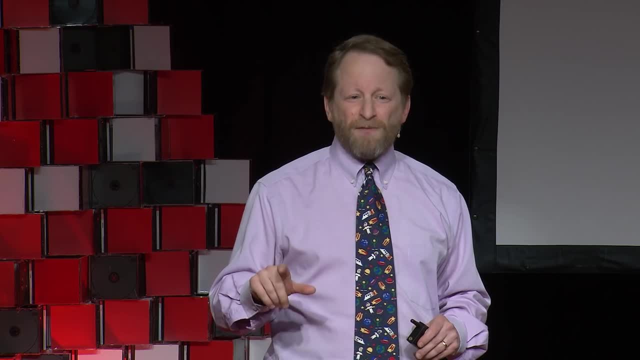 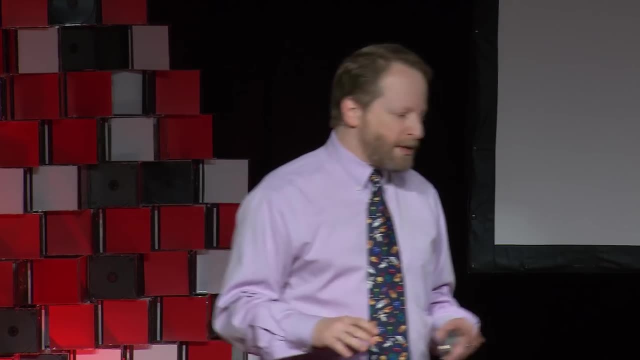 You know what the worst thing in the world is- Being in a school bus with 45-year-olds who are angry. You know what's worse than that? Nothing. So we brought them back to our school and someone in our faculty who was far smarter than I. 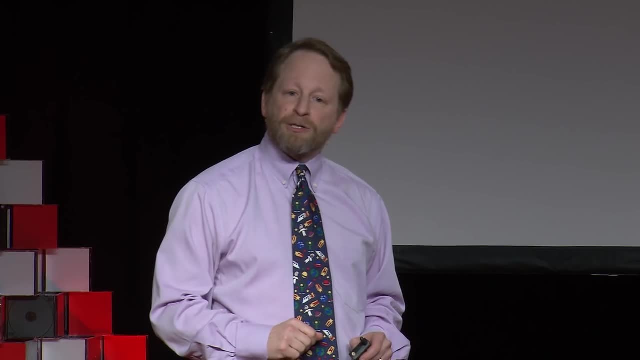 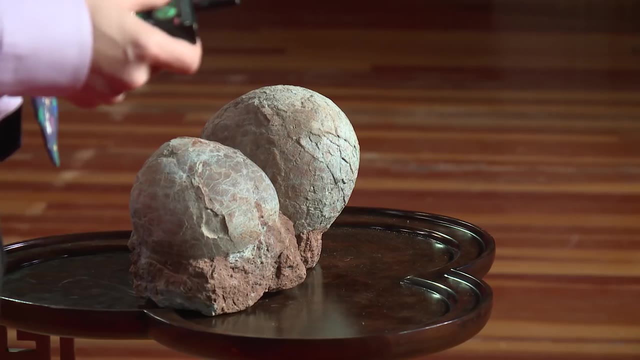 went to the display case and took out our real collection, which included some hadrosaur eggs. These are roughly a little less than 100 million years old and they're real. So we let our students actually touch the real dinosaur eggs. They felt like magic. 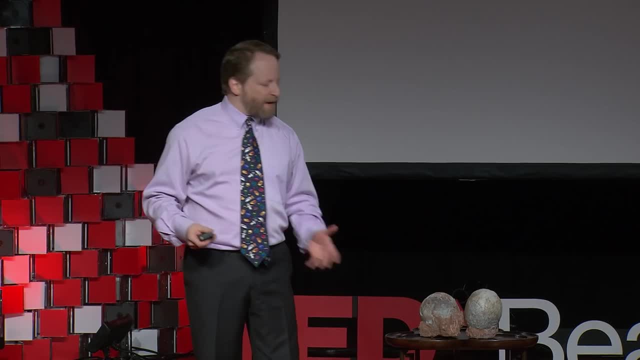 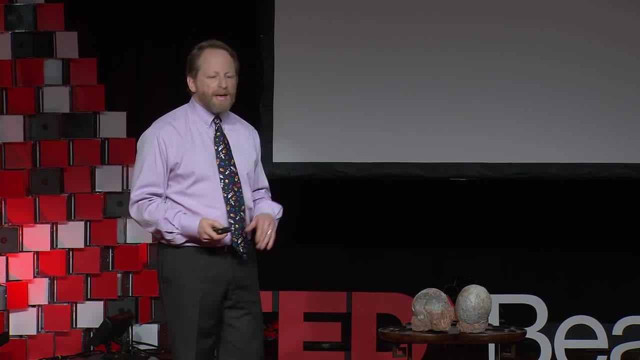 They reconnected with the science. Instead of being angry or frustrated or feeling cheated, they felt reconnected. And, by the way, that desire to connect with an object or an event or something in your classroom is not just for children, For example, it's with adults as well. 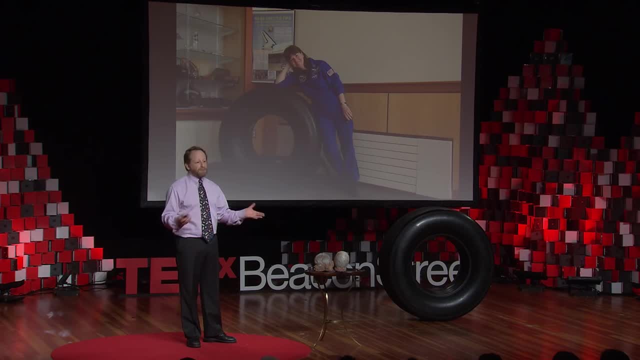 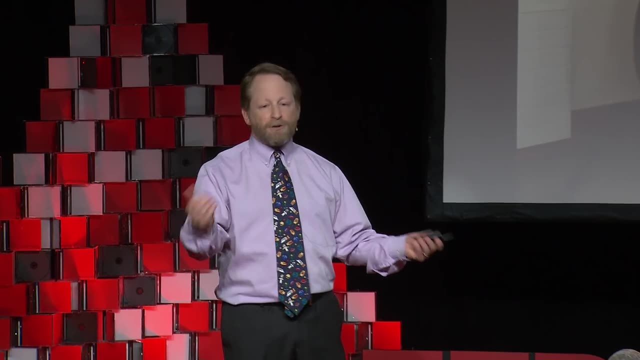 On the stage with me. here I have a genuine tire from the United States Space Shuttle. It was from the Columbia Space Shuttle. We had an astronaut, Katie Coleman, come visit our school and give one of those, and it was really exciting. She was on her way out. 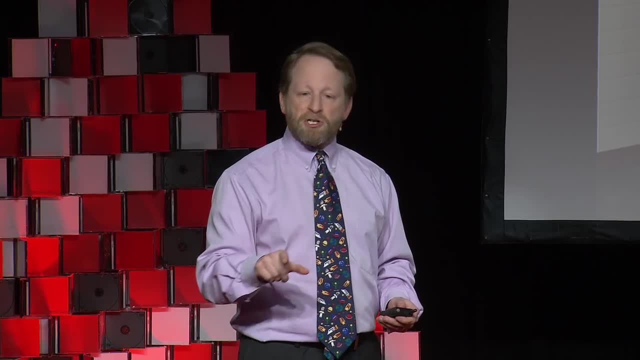 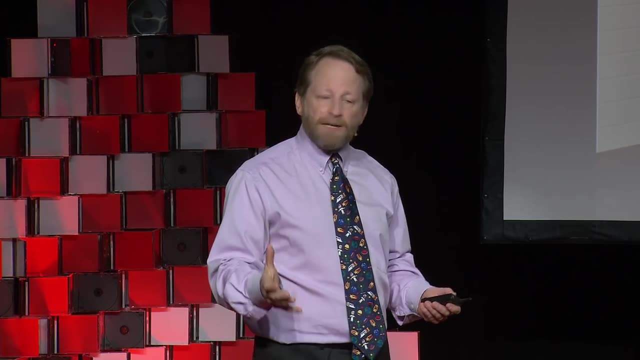 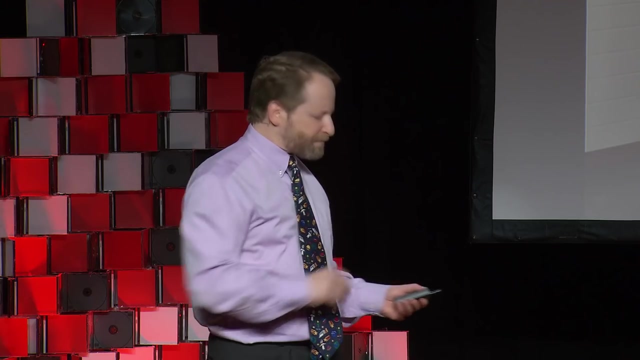 saw this space shuttle tire which we have for outreach, found out it was a tire from her space shuttle mission and ran across the lobby and gave it a giant hug. She actually was really excited about being reunited with her space shuttle tire. She insisted that I take this space selfie picture. 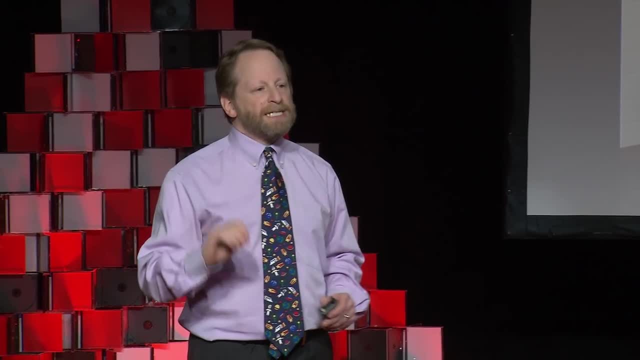 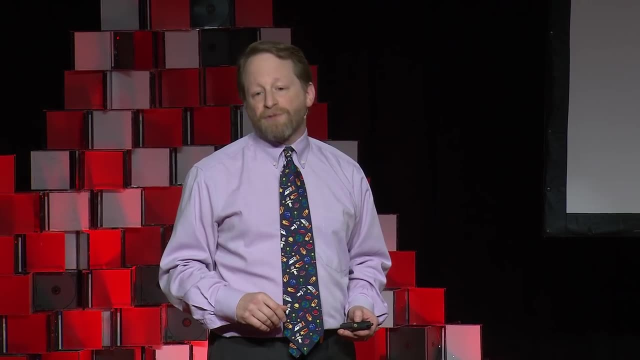 so I did. But it reminds us that this desire to connect with things- not just in science, but to really connect with things- is a human thing. It's not just for children, it's for adults as well. So what I learned we do well in schools. 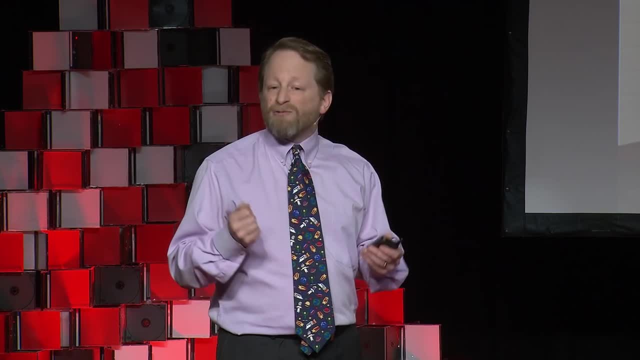 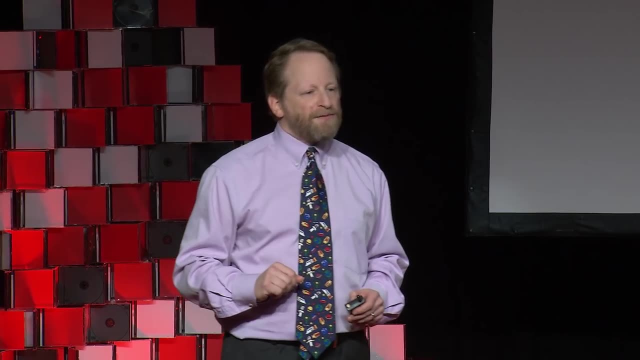 at a very young age especially, is to do hands-on work that really connects students with real science. Now, what I found out, what we don't do so well, is not really an artifact of how we teach science. it's an artifact of you and me. 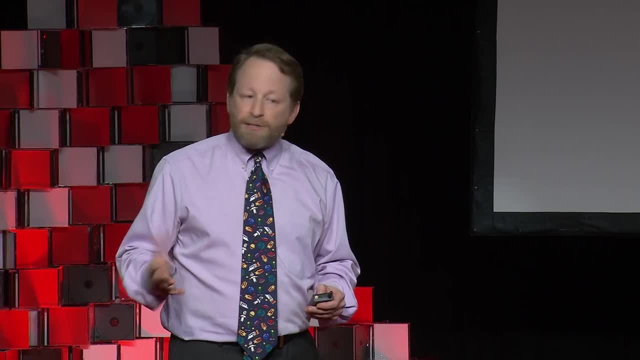 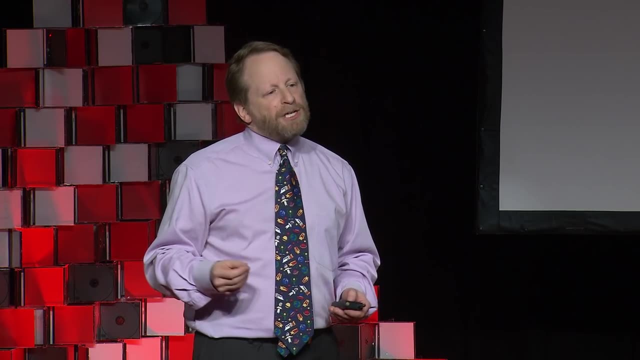 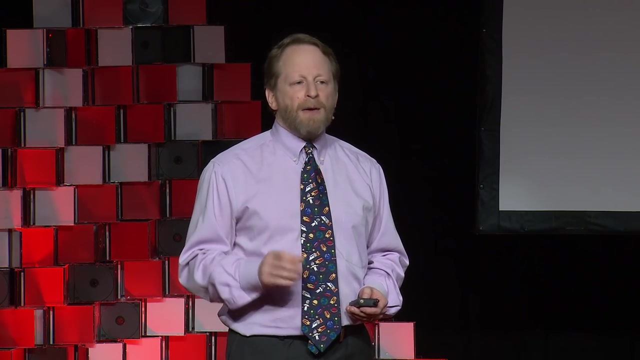 and our human brains. Scientists, you all have human brains, right I was checking. Scientists use a lot of numbers and that actually can be very alienating for children and adults. In fact, in my work I find a lot of adults are afraid of science. 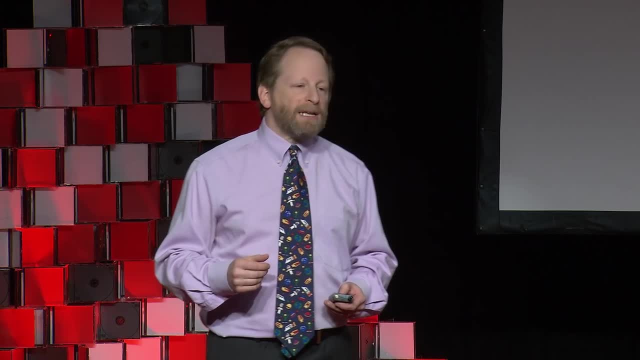 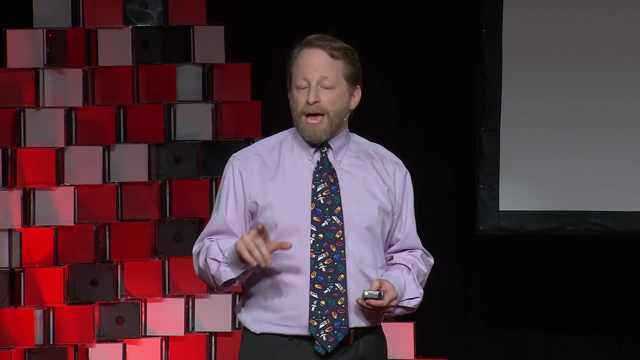 because they think if a number like a billion comes up in a class, that they should understand it. Well, if you understand what a billion is viscerally, that makes you abnormal. Most people don't understand large numbers. I'll give you an example. 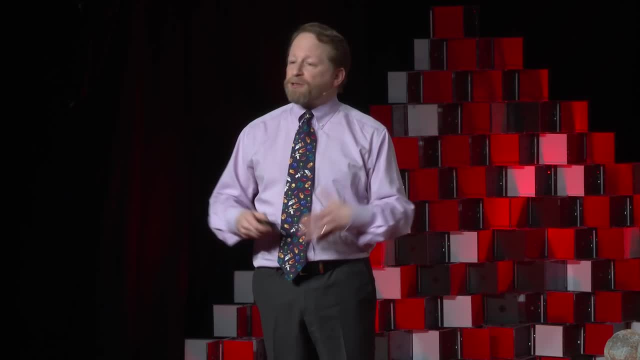 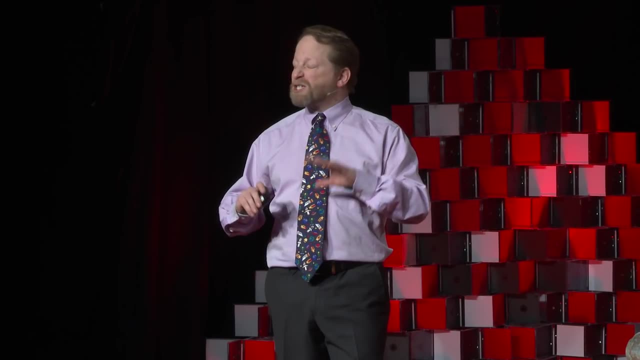 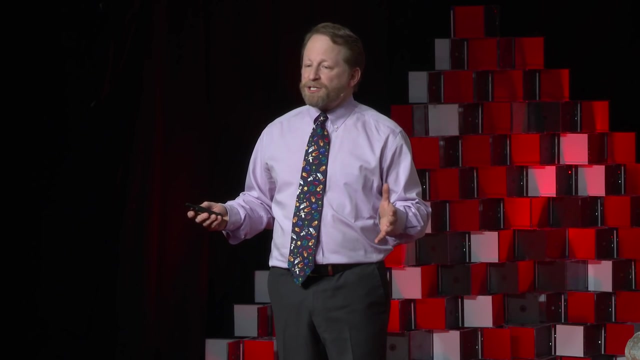 I teach astronomy and I was giving a lecture in the solar system and I said- and this is true, so don't get scared- in about four and a half billion years, the sun's going to explode. the earth will be gone. 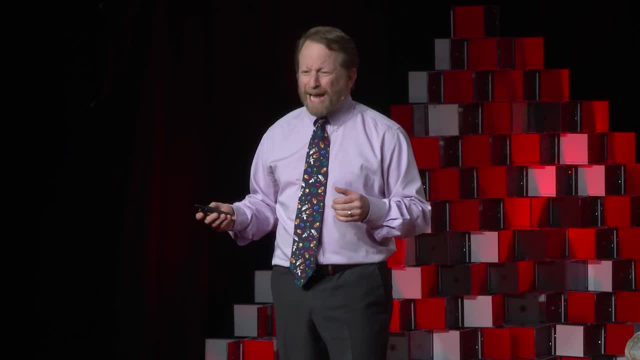 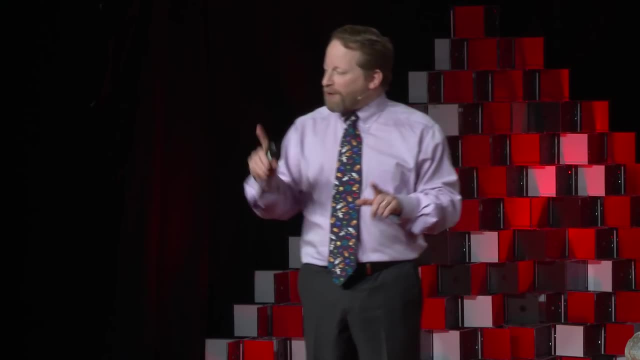 end of the solar system. A woman came up after my presentation, really upset, and she said: are you kidding me? Is the earth going to be gone in four and a half million years? I said no, four and a half billion. 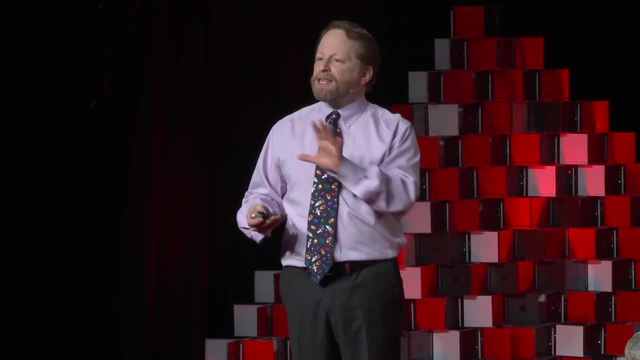 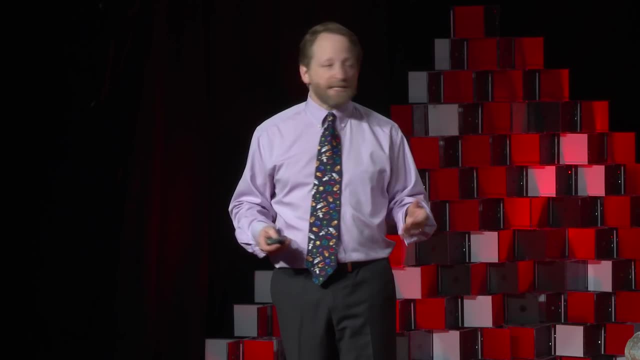 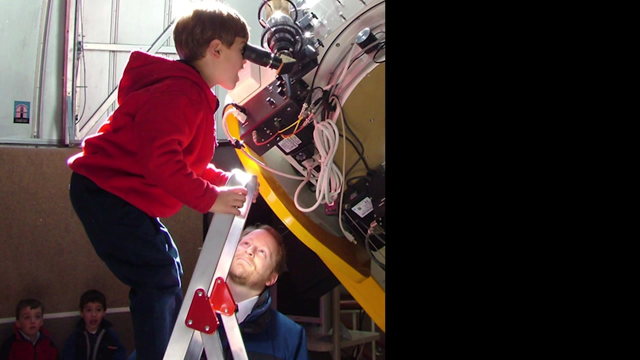 The idea is: if you don't understand numbers, that makes you normal, not dumb. And scientists have this difficulty in that it involves large numbers and distances, especially in astronomy. So at our school we have a large telescope. we do a lot of science. 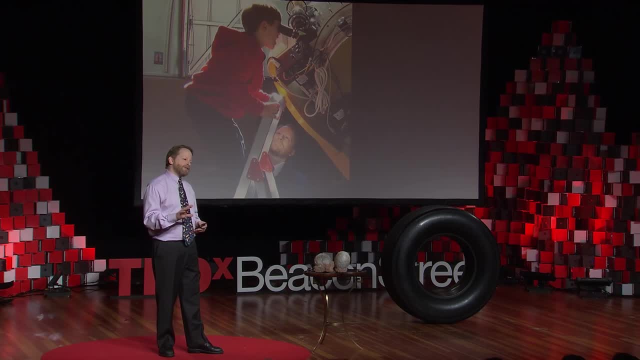 and we try to make it as hands-on as possible. So here's how we do it. We actually have kindergarten students who've never looked through a telescope. look at the sun with a safe filter on it. I promise you Exploding off of the sun. 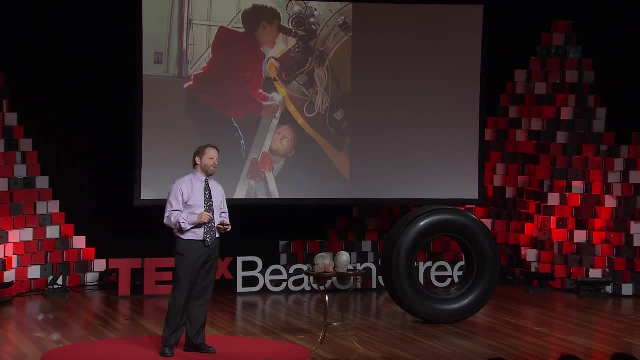 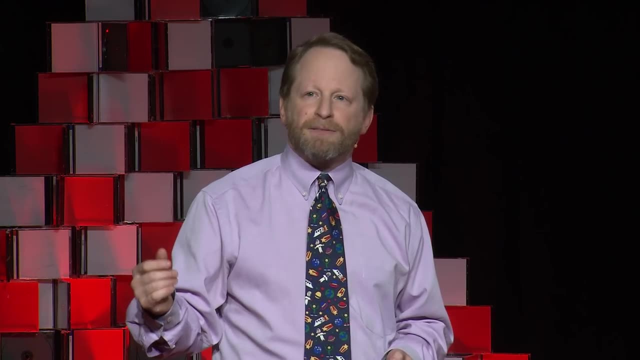 That's pretty exciting stuff. But before we do that, we make them do a little bit of work. We ask them to make a drawing of what they think the sun is going to look like first. That's what scientists do. They make predictions. 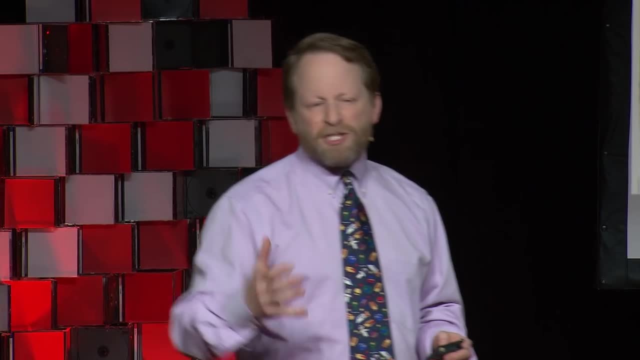 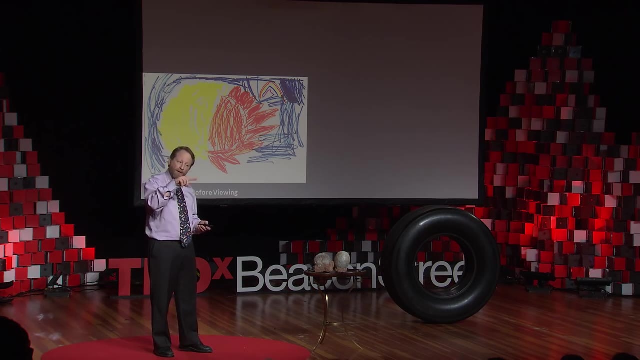 So, for example, this particular student, four years old, almost five, wasn't sure whether the sun would be red or yellow, whether it would have flames on it or not. This kid's an optimist. got a little rainbow going on there. 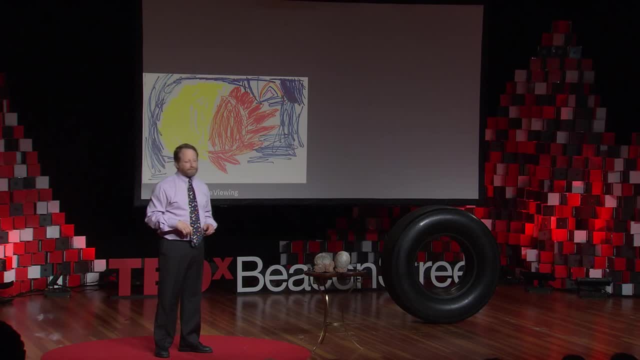 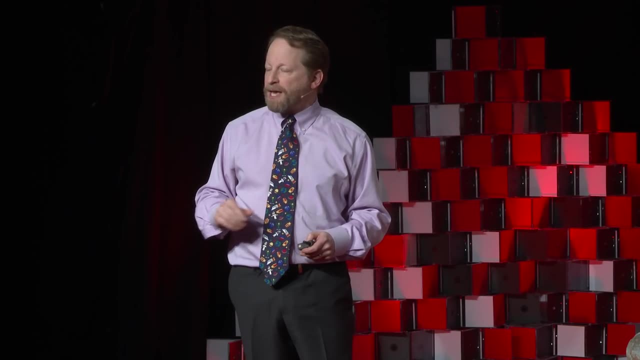 Got a blue square all around it watches too much television. So the way it works is this: These students have preconceptions. You might call it a hypothesis. if you're a scientist, Then we let them look through the telescope at age four. 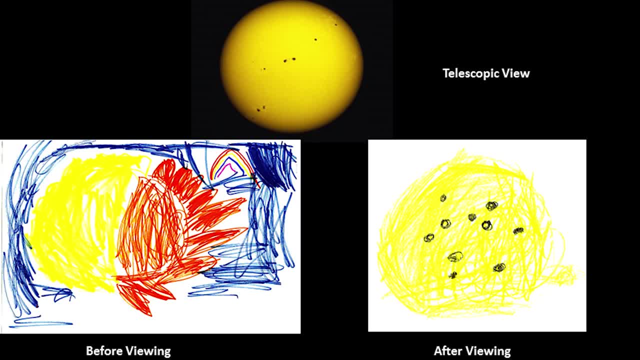 and they see it's not like what they expected, And then they make a second drawing. So in science we actually call it a hypothesis, observation, recording of data. This is science from a four-year-old point of view And I've got to tell you. 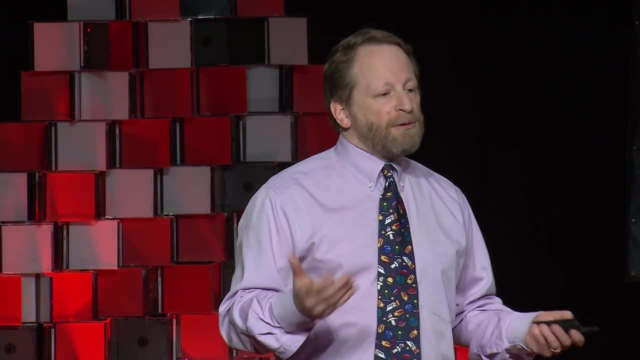 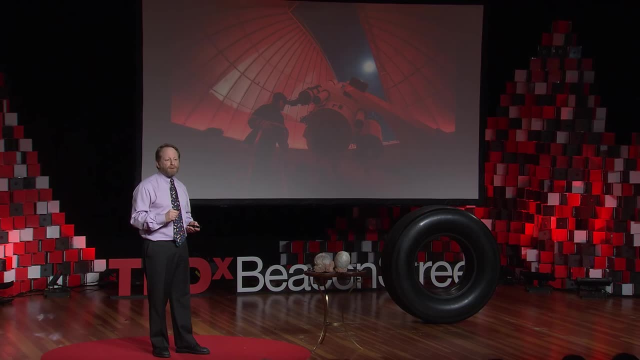 you can too. We try to involve our students in hands-on experiences which, as you know, really help in the learning process. Instead of looking at a picture of the moon in a book, why not look at the real moon? Fourth and fifth grade. 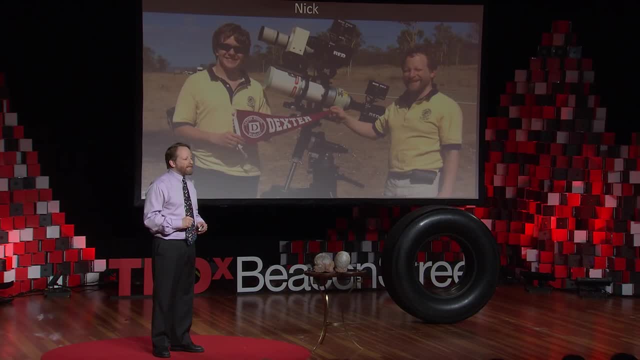 they can even take pictures of the moon. We've had students who want to learn more about astronomy. This is Nick At age 17,. he came with me to Australia and we photographed a solar eclipse- And what's nice about that? 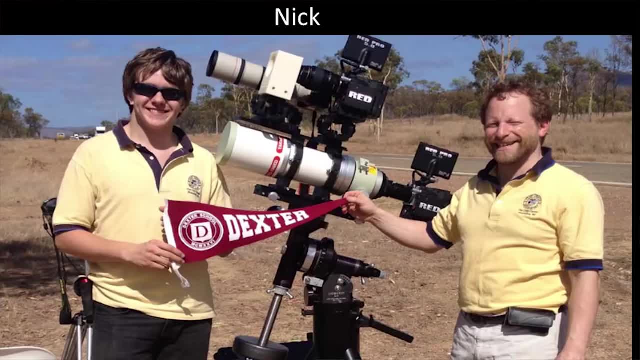 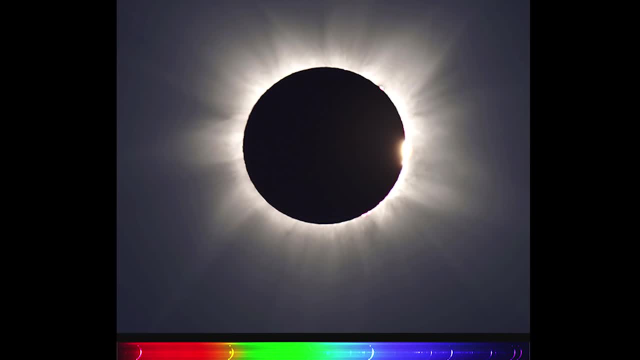 all the equipment you see there. it's in our lab. There's a small yellow box at the top. He designed it, printed it up on a 3D printer and took this picture with him. Thirty seconds after that eclipse, he said to me: 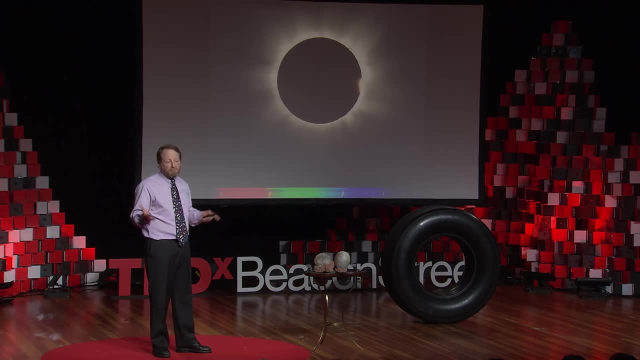 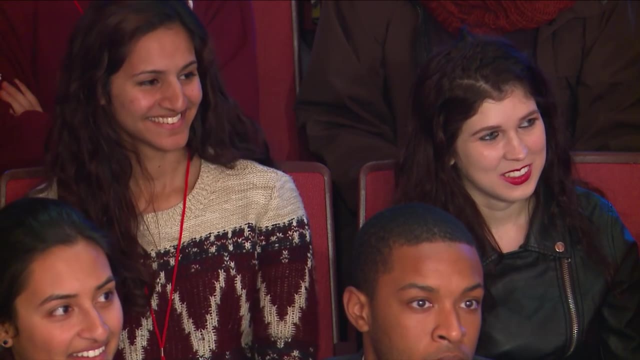 I want to do this for a living. I didn't want to tell him living, but he wants to do it for a vocation is what he meant. So we have students doing things that professional astronomers never dreamed they would do at that age. 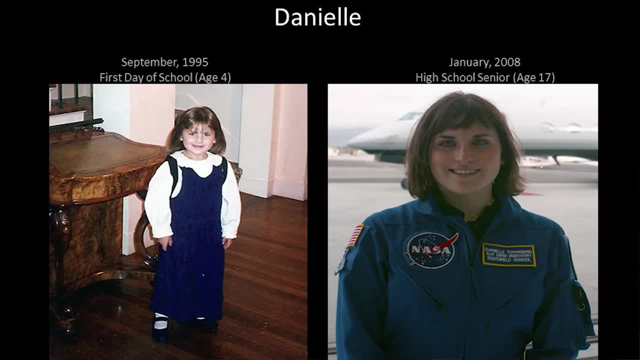 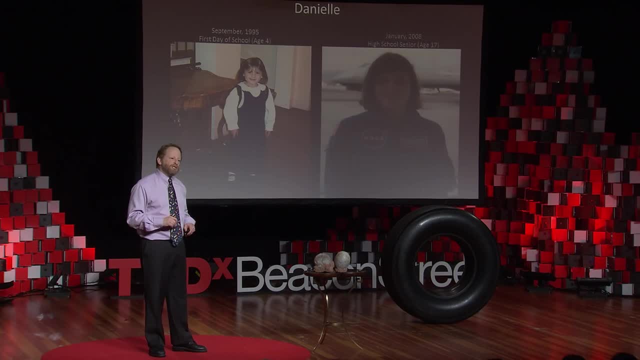 This one. this is a great picture of Danielle her first day of school age four. When you work with students at a young age, they don't know they shouldn't be doing all this great stuff When she was in 12th grade. 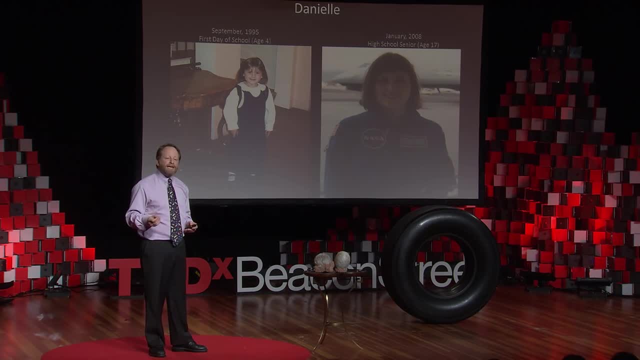 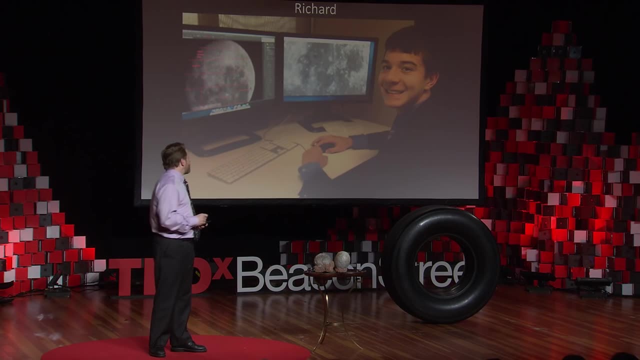 she joined me on a NASA flight over the North Pole and we photographed the aurora and meteors. Danielle's pictures of meteors were better than the ones NASA had. This is Richard. He graduated last year. He's currently in an Ivy League school. 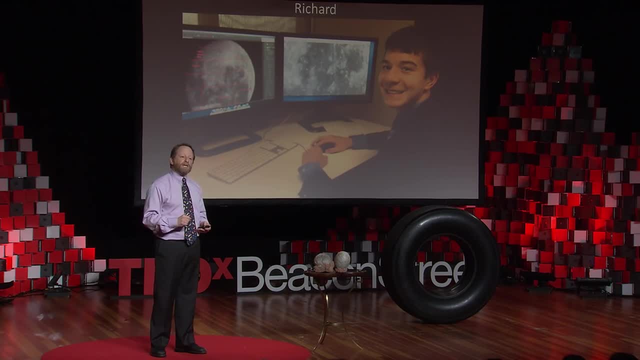 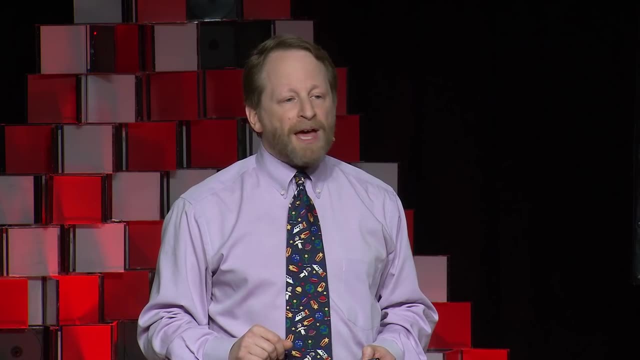 studying biology Doesn't like astronomy. Working on one picture of the moon, He called it the Mega Moon Project. That picture, you see there, is built of 4,712 little tiny pictures of craters. He stitched it together like a mosaic. 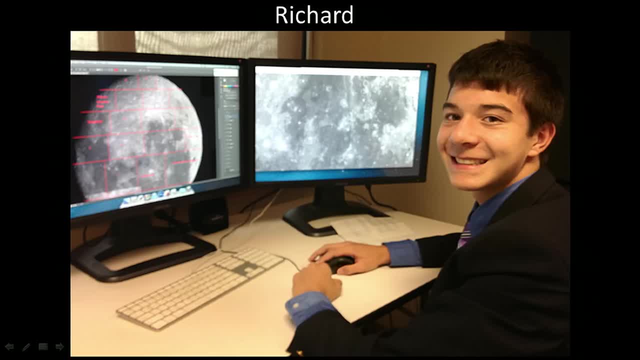 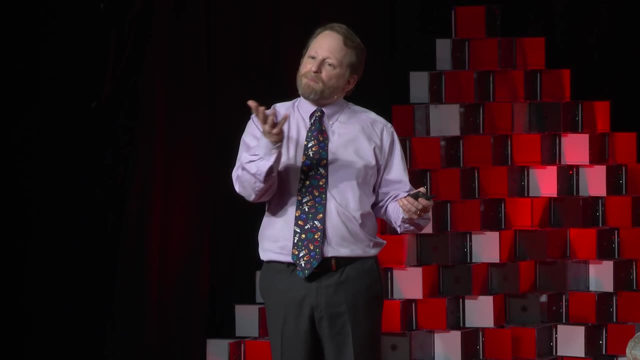 He did that because he was interested in learning how to do that technique. Although he's not interested so much in astronomy, he's interested in biology. In his junior year there was an application for scientists. They need scientists to study the neurons in the brain and follow around. 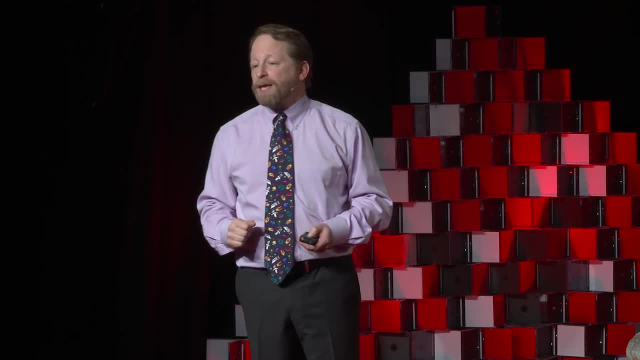 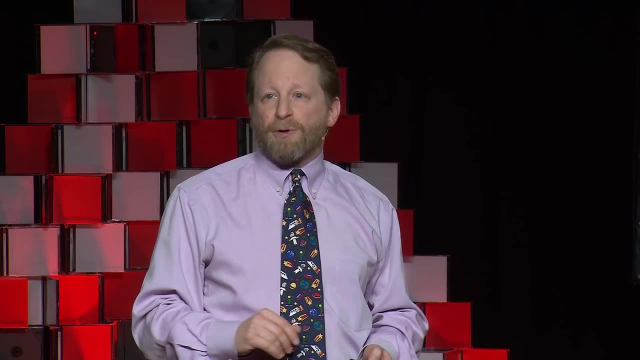 the neurons through the brain. Guess what? He got the job. Now he goes to that school, So you never know what skills you're going to use. Astronomy is really a lot of fun, no matter what you do. This is one of my final slides. 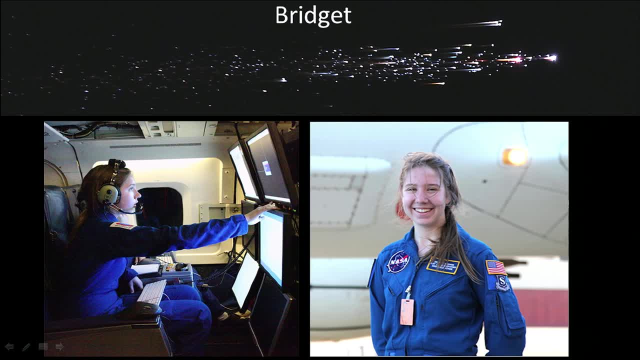 This is Bridget At age 16,. after coming through all of our astronomy programs and learning how to do hands-on science, she was the youngest person to join a NASA flight crew And took images of reentering spacecraft, which you can see right above that. 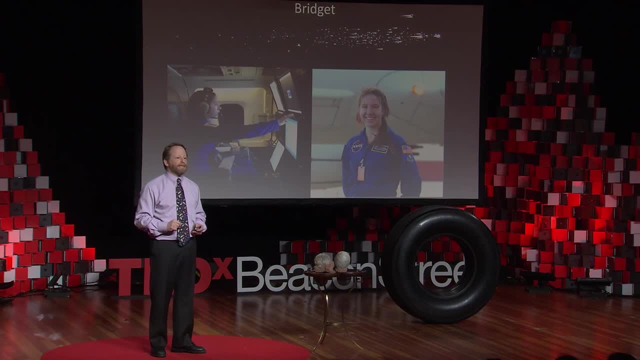 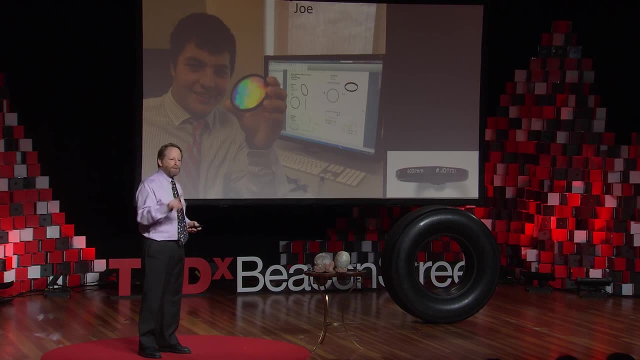 Those are her images. It's pretty exciting for a 16-year-old. I kind of feel like an underachiever actually. You know we have a number of students which I won't tell you about, but this one's special. 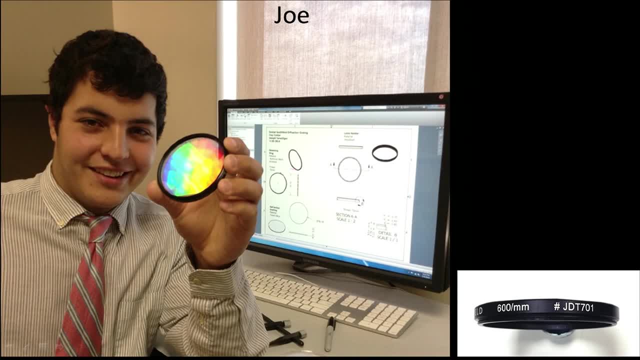 This is Joe. Joe was studying engineering at Worcester Polytech this year. He started doing some really interesting work in engineering and we gave him an opportunity. When students take an opportunity, they really sink in because, again, they don't know they really shouldn't. 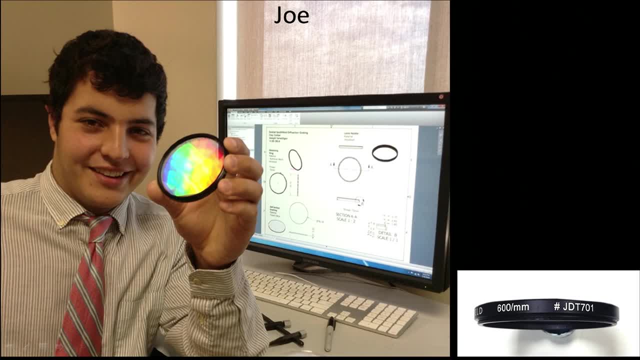 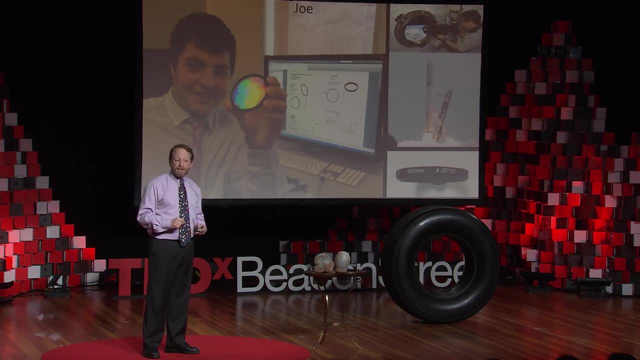 be doing these things. Joe designed a part that's now up on the space station- That lens that you see. there is called a diffraction grating. It was launched on Elon Musk's SpaceX rocket, docked up to the space station, and now when astronomers take pictures. 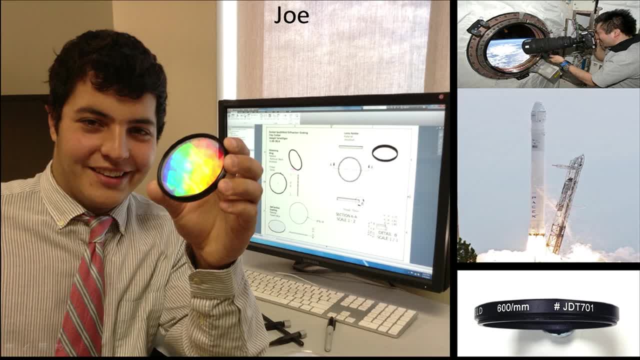 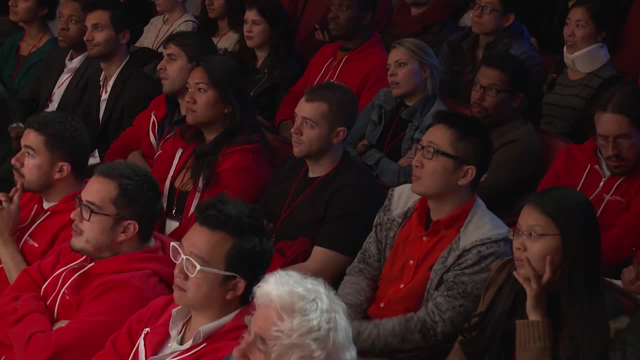 out the window and they want that kind of lens. they're using Joe's lens, But I'll tell you something special. Always tell a student you appreciate him or her. See the serial number in the lower right: JDT701?. First it was 701,. 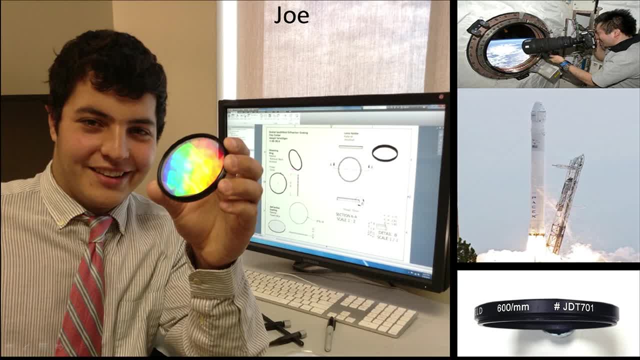 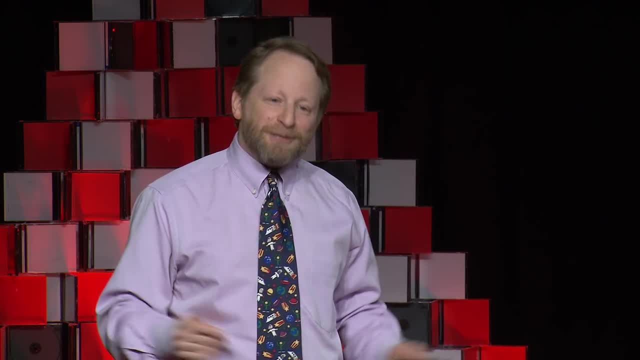 then NASA said we need six characters, so we just put his initials on it. So that's right, we tagged the space station with Joe's initials. It's kind of special. Not everybody can say that. So the last couple of pictures. 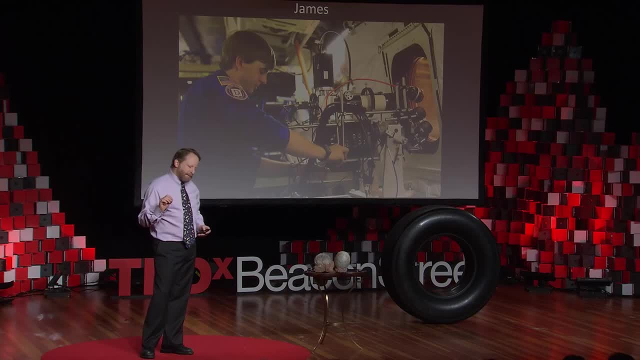 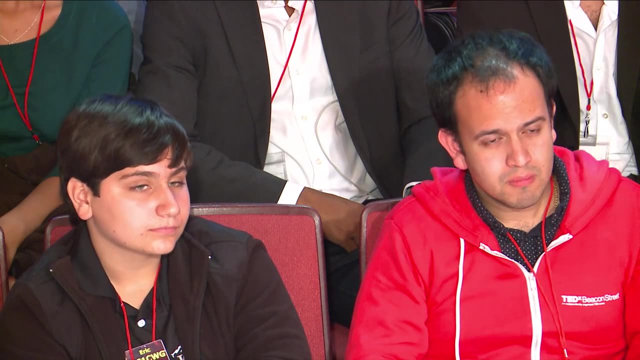 I have are kind of interesting too. I want to get across to you the importance of having a student actually do the work. The device you see there was designed and built by students. I did almost nothing. What that means is, when we use it, the students have. 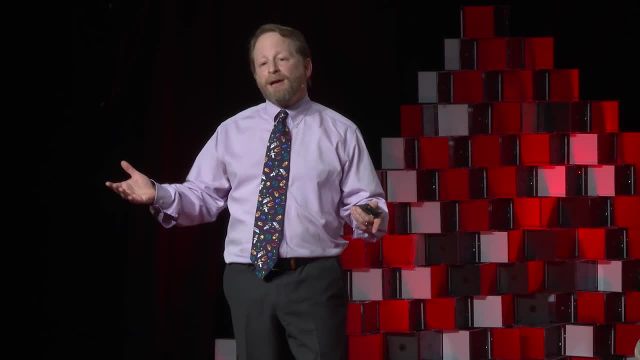 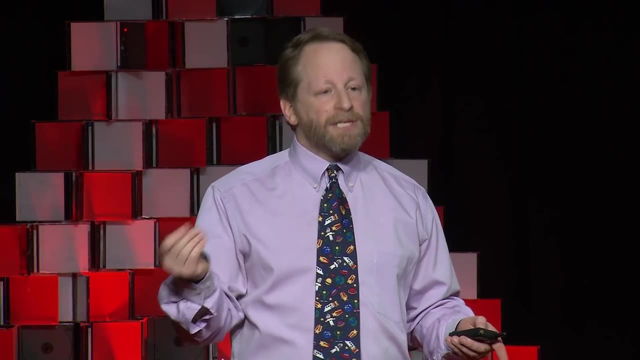 ownership over it. They really did it themselves. If I come up there and yank a wire out, which I don't do that much, that student doesn't say, Mr Danowitz, it doesn't work. They'll say, oh, this is loose, and they fix it. 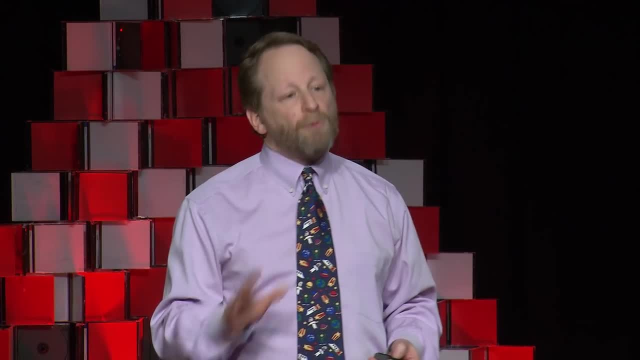 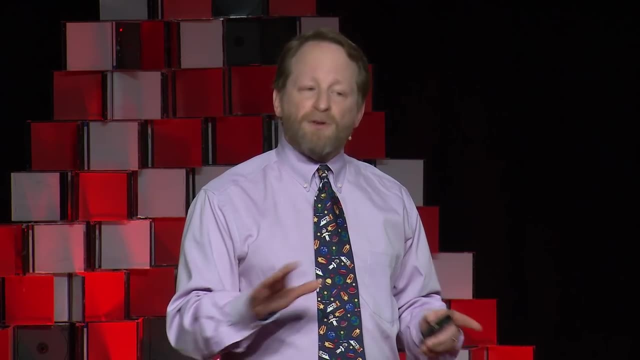 Because they know how it works and they're confident because they're the ones who did it. So the last slide I have for you is very special. I just arrived a few hours ago from Dubai in the United Arab Emirates. I was in the UAE this morning. 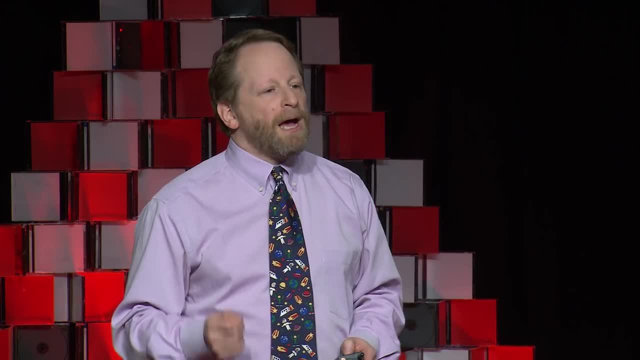 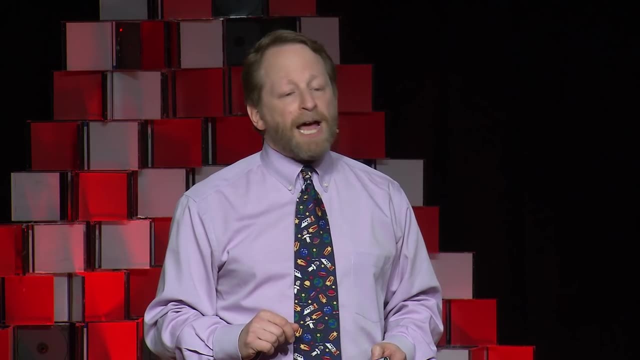 So if I look a little tired, what can I say? I just brought a student with me on a European Space Agency and NASA mission. In case you didn't know, a few weeks ago an asteroid was discovered on impact course with the Earth. 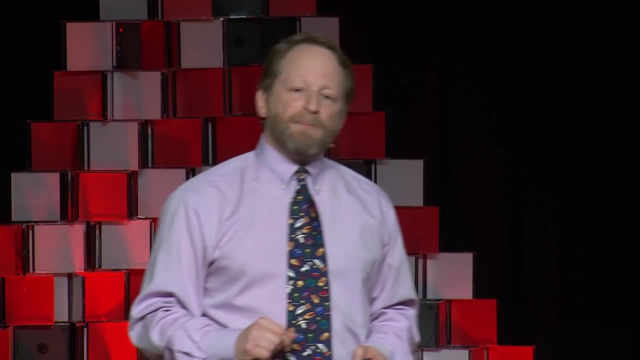 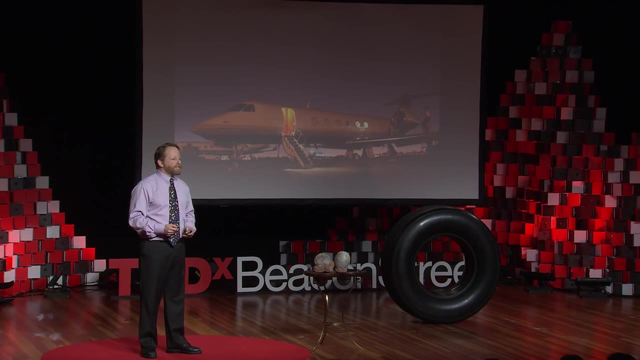 That asteroid was set to impact the Indian Ocean the day before yesterday and it did it and we were there. NASA wanted to get some images of it, so they called on our school and I said we could go if we brought a student, which we did. 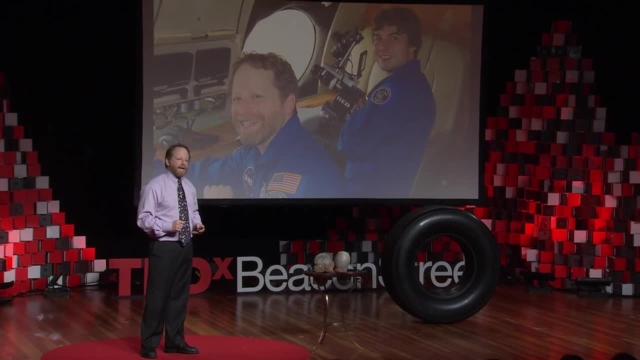 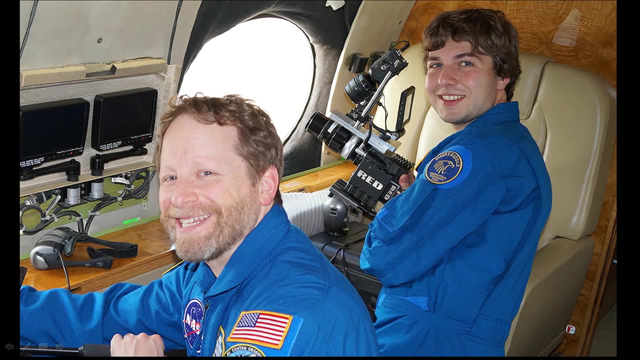 So here's the way it worked. I actually brought a student of ours out- This was about 18, 20 hours ago- on a high altitude jet over the Indian Ocean, What? It seems strange to you- Students do these things. So we did rendezvous with the asteroid. 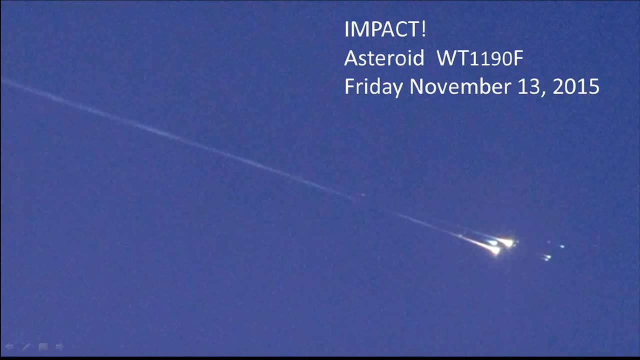 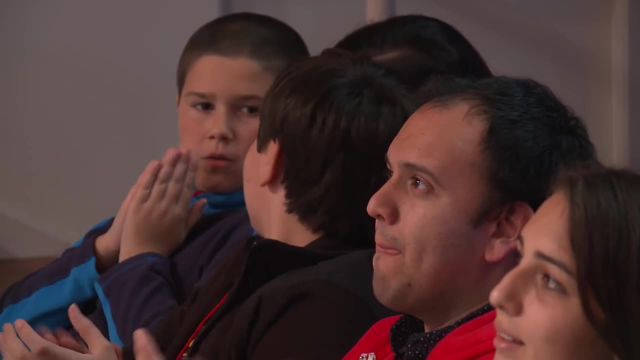 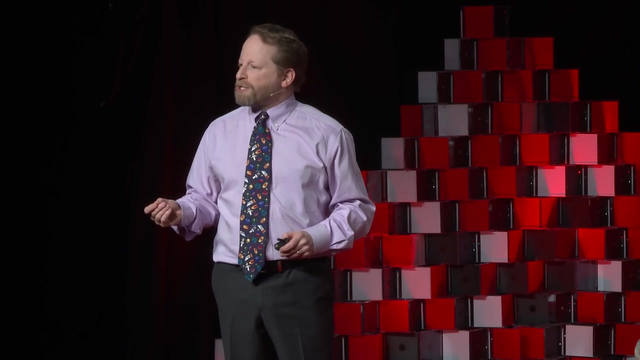 It did hit, and here's the first picture of it, just taken a few hours ago. You're among the first to see it. A few parts of that are really remarkable. The student part is great because it's our responsibility to mentor these students. but you know what? 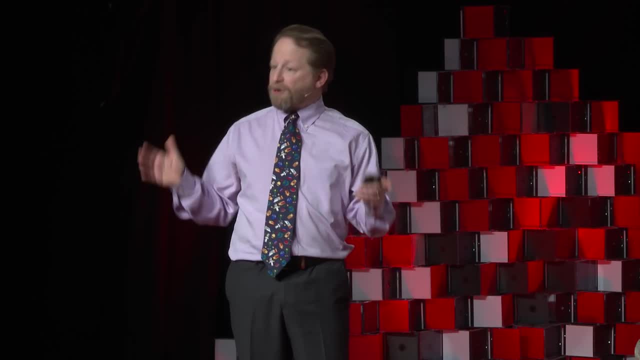 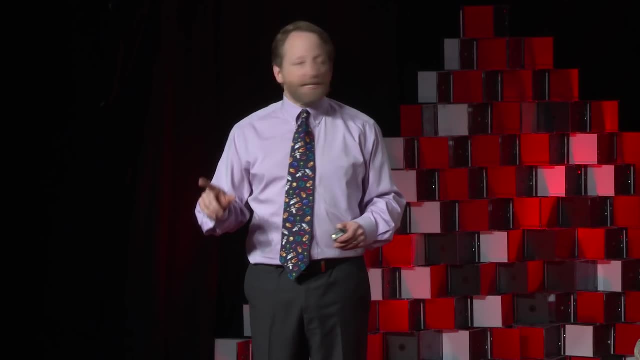 I had a student really feel good about flying out to where there was an asteroid going to impact. The asteroid hit on Friday the 13th. just a coincidence, It's true. The computer assigned it a name: WT 1190F. 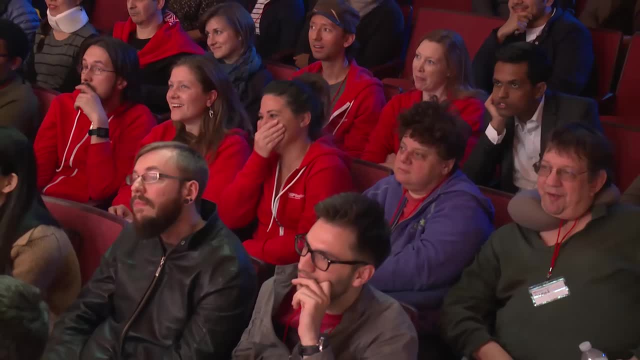 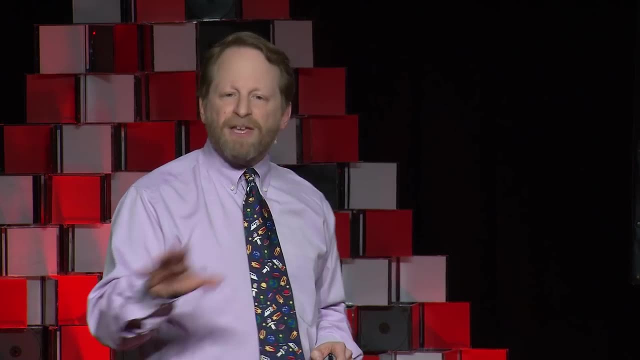 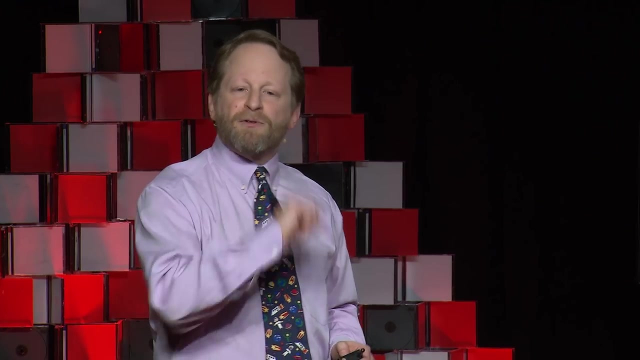 Strange but true. Look, I know I get it. Students in the audience. The idea is: these things happen and to make the most of them educationally, we have to have students that are ready to go. So what can I say? I'll leave you with two points. 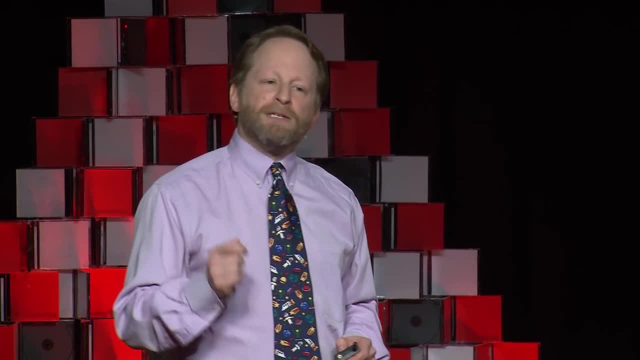 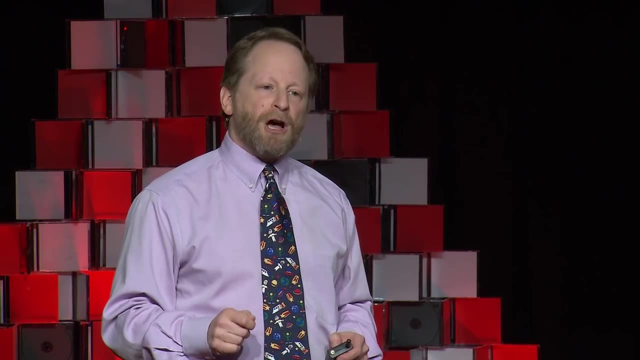 Number one. one of the most important things we can do is teach students well, Because when we're teaching, we're training our replacements, so we better do a good job And finally take this home with you if a four year old can do science. 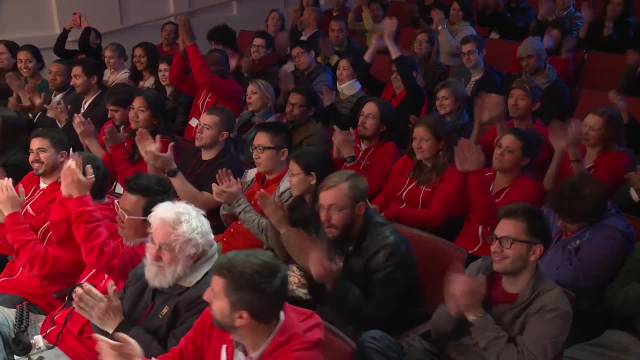 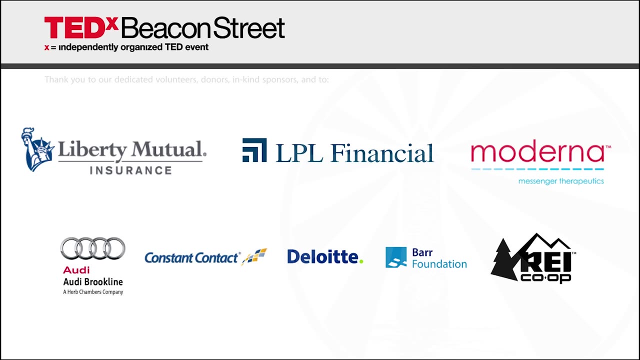 you can too. Thank you, Music.